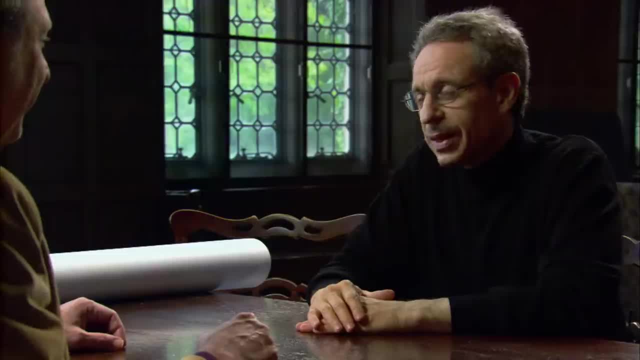 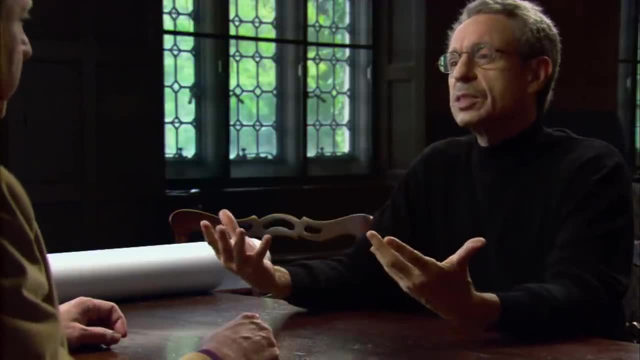 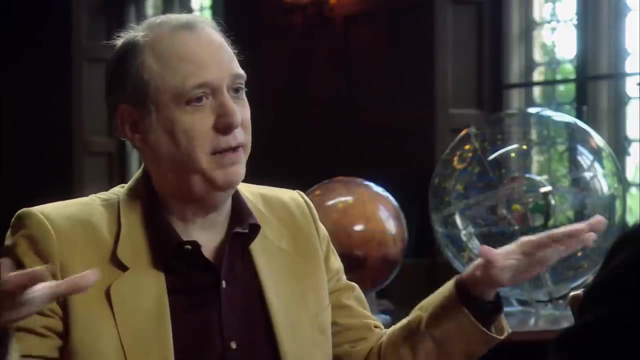 maybe 10 to the minus 35 seconds after the beginning. That's it. It's incredible, It's an incomprehensible period of time. What happened during that period of time results in this enormity that we see today? Because the universe has expanded so much. these microscopic small things have expanded to very large scales by the present day. 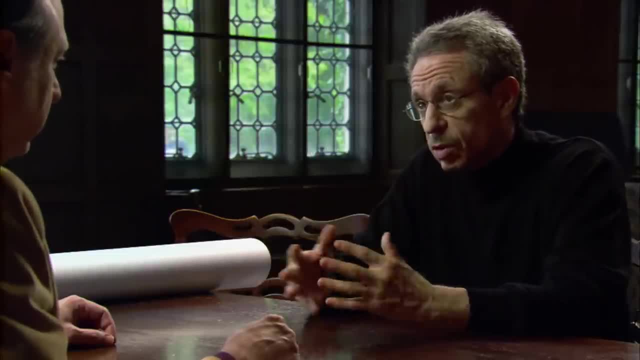 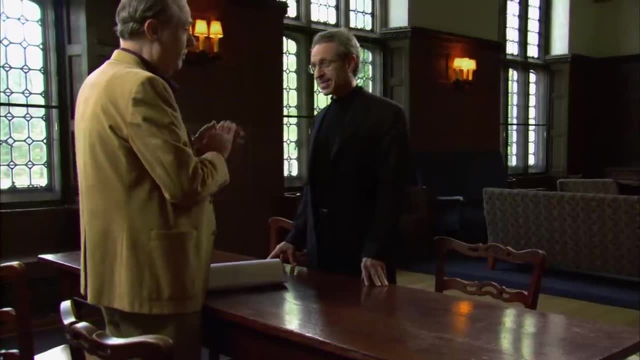 How can we begin to understand some of the rich detail of this structure? Well, let's look at a map. Okay, Okay, Okay. well, this is a map of the entire universe, All of it, From the center of the Earth, all the way out to the furthest thing that we can see. 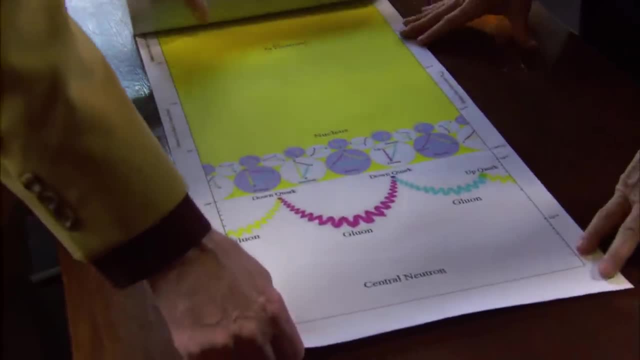 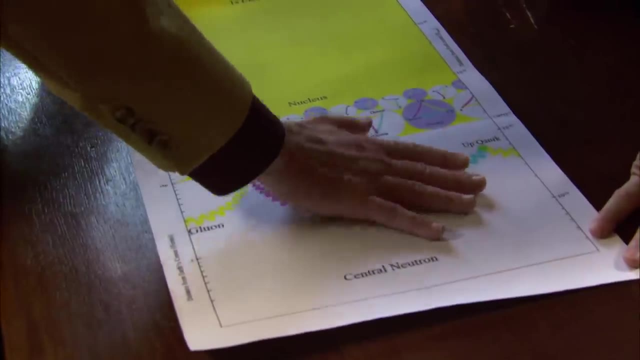 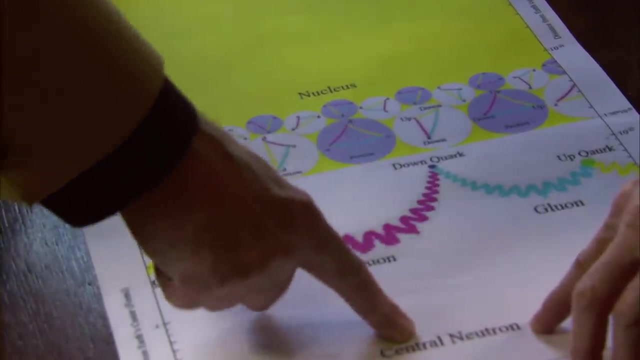 Okay, So it starts out here with. the center of the Earth is iron, And this is the central iron atom. This is the nucleus of the central iron atom at the center of the Earth And this is the central neutron in the center of the iron atom. 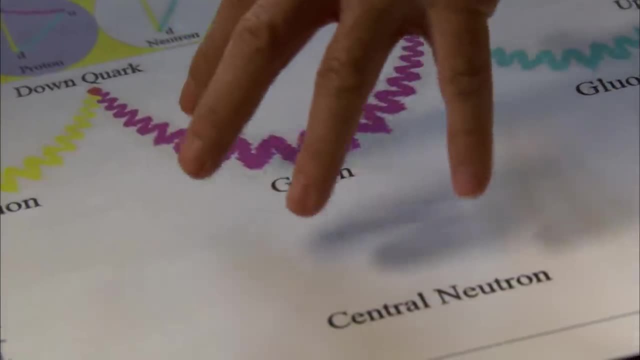 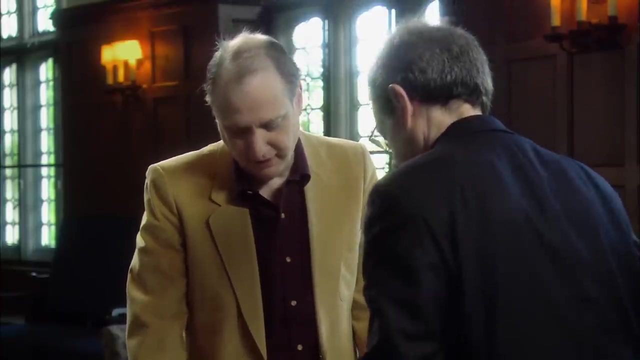 And we can see the three quarks. So this is just the neutron in the central atom, in the center of the Earth. That's right, That's right, That's right. And so we have a neutron here, We have a proton here. 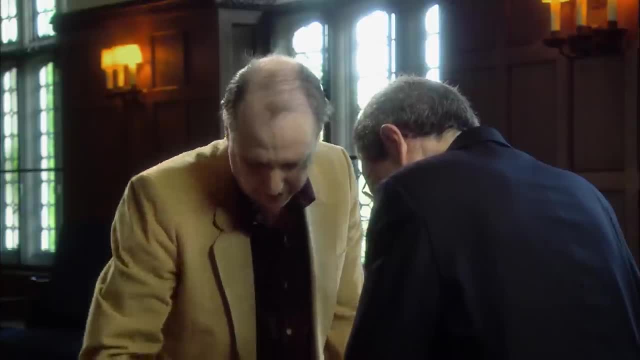 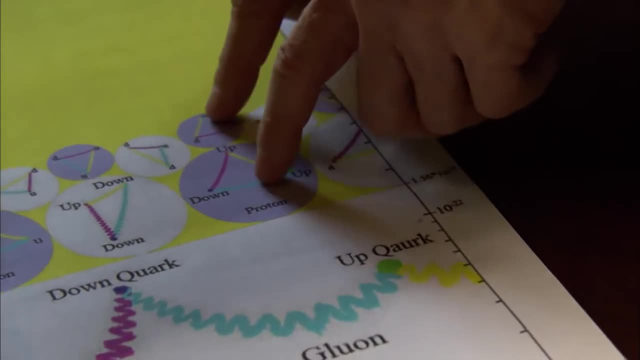 Neutrons. here We're showing an equatorial slice. Each tick mark over here is a factor of 10 further out, So it's a logarithmic scale. It's a logarithmic scale And so, even though these look different size, these are in fact the same size as the scale changes. 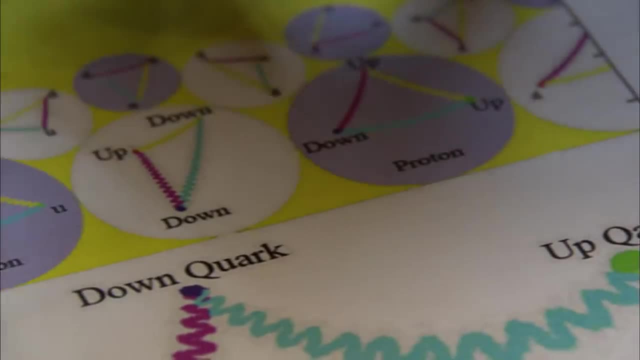 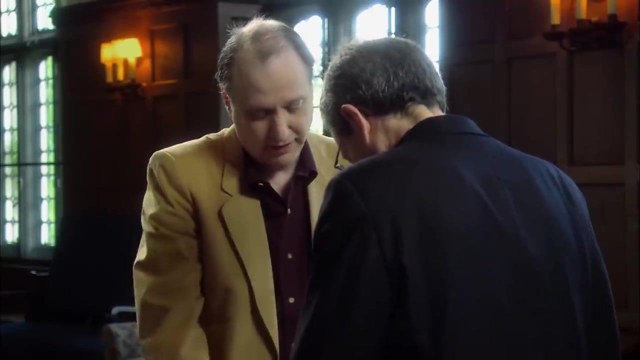 Yes, Every time the scale, every time the distance goes up by a factor of 10, the scale goes down by a factor of 10.. So things that are further away are shown smaller. This allows us to do this, To get the whole universe in it. 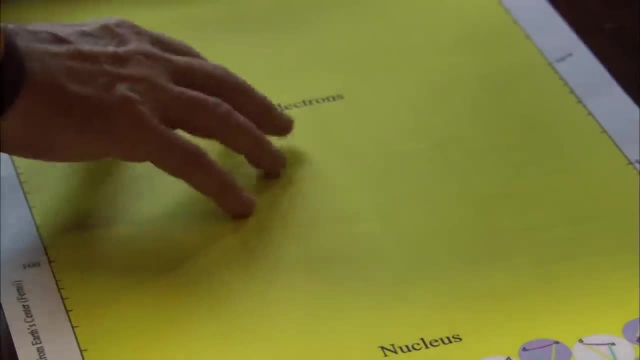 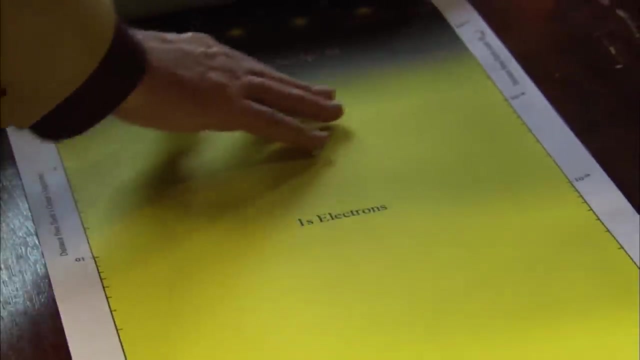 To get the whole universe. Now we come out here. This is the innermost electron cloud Still in one atom of iron, In one atom of iron, And here's the outer electrons. And then we come out and we see the other iron atoms. 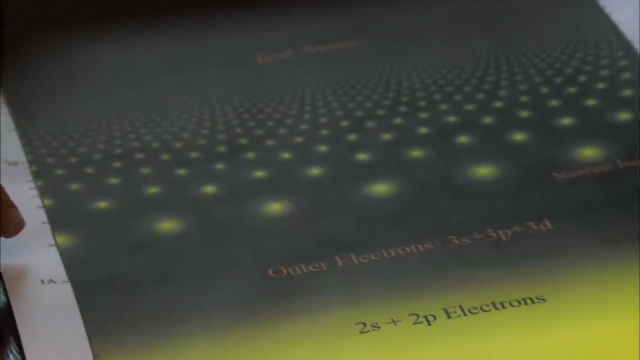 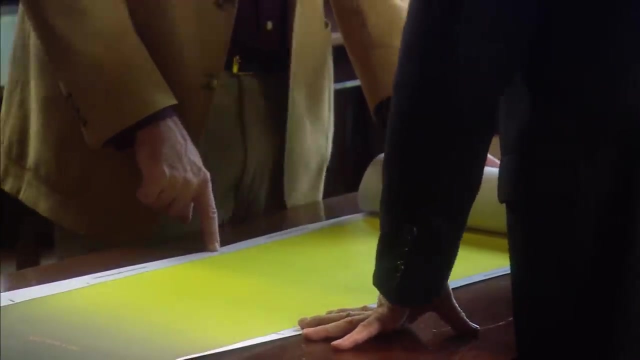 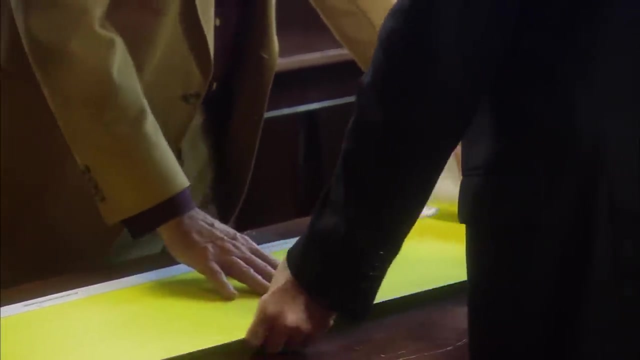 And they're in their crystal structure here And now. we're one millimeter away from the center of the Earth Right, And so we're still in the solid iron core of the Earth. Each one of these is a factor of 10.. 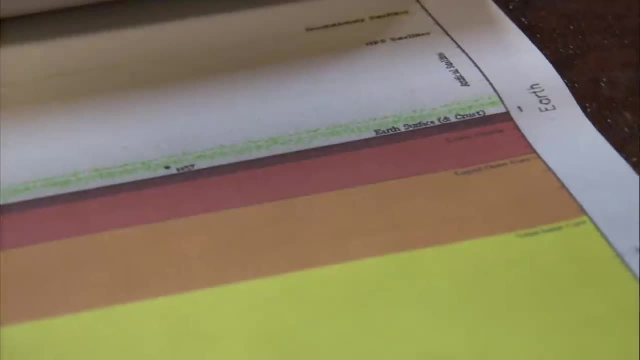 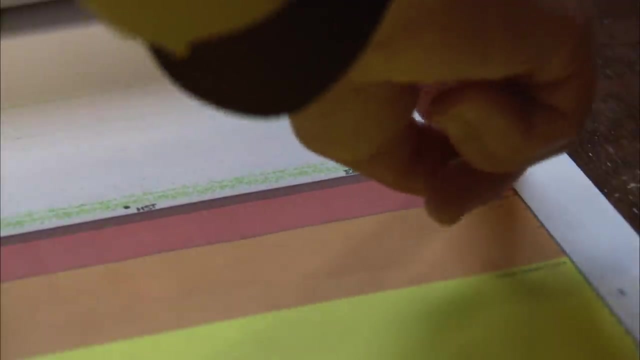 And finally we come out. Here's the outer edge of the solid inner core of the Earth And here's the liquid outer core, And here's the lower mantle and the upper mantle, And this is the surface of the Earth at the Earth's equator. 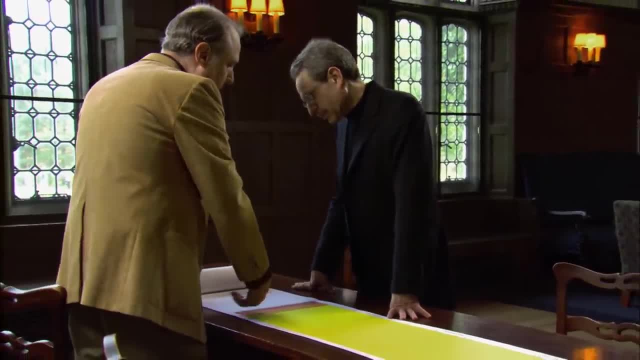 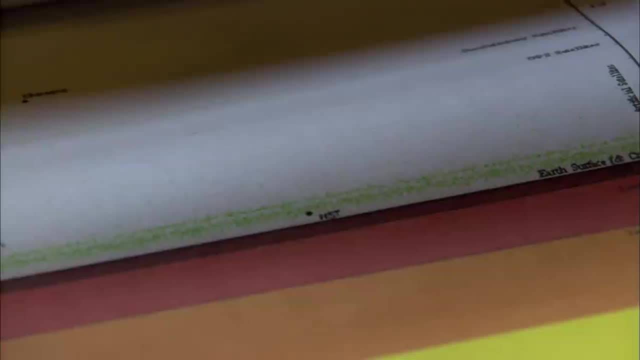 And this is showing you a 360 degree panorama looking out. And again, this is 10 times. This is 10 times the radius of the Earth. We can see here all the Earth's satellites. There's about 8,000 artificial satellites. 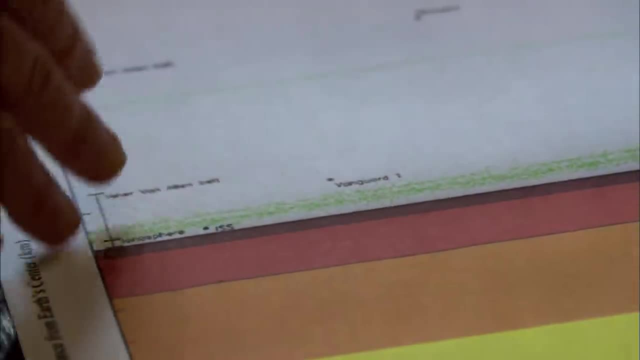 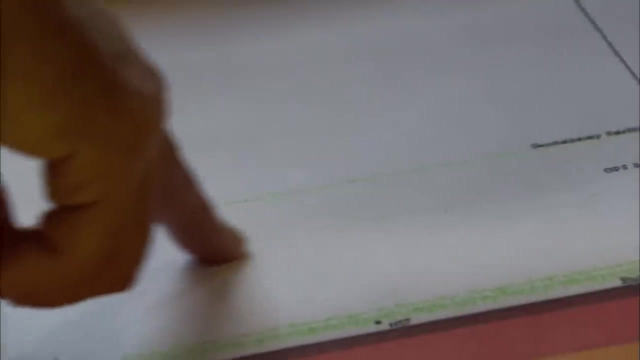 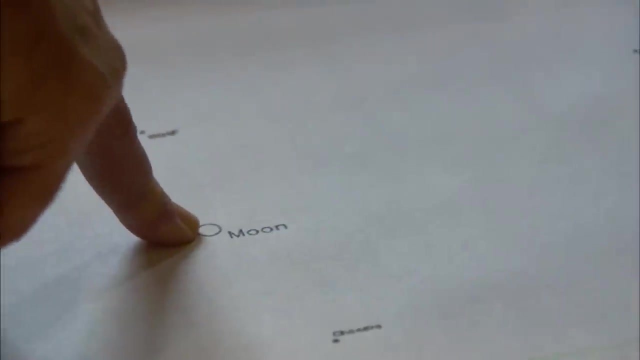 You can see the International Space Station here. Here's the Hubble Space Telescope. These are in very low Earth orbit And here are our GPS satellites that you use. And then we come on out here We get the moon. This is about 60 Earth radii away. 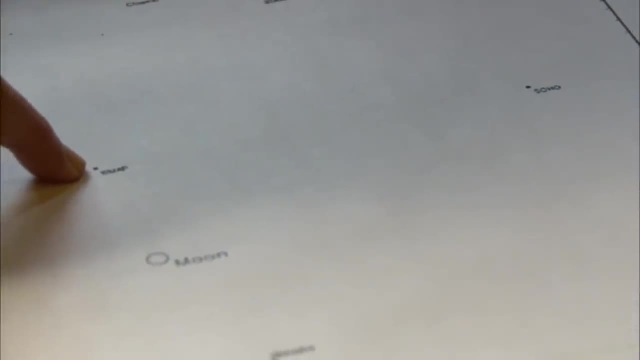 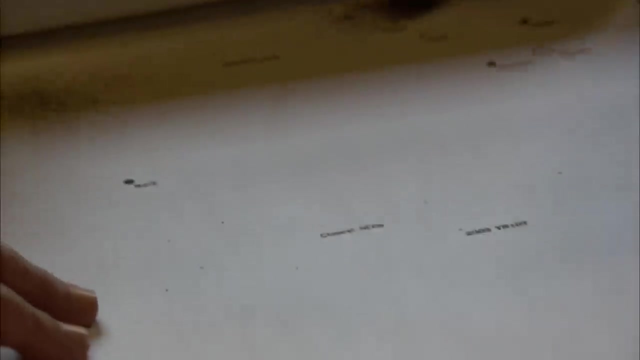 And here's the WMAP satellite. This is observed. the cosmic microwave background radiation from the early universe. We get some near Earth asteroids here, And here's Mars. And how many Earth radii is that? Well, this is getting up to 10, to the fourth. 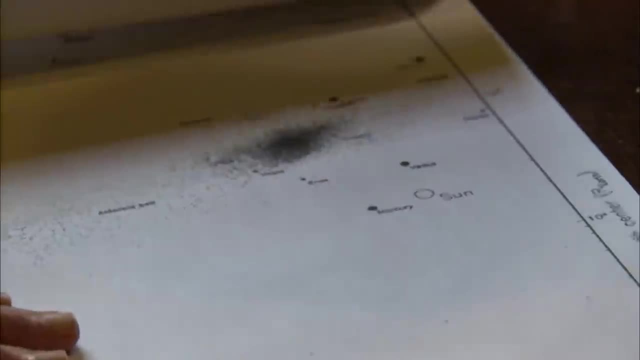 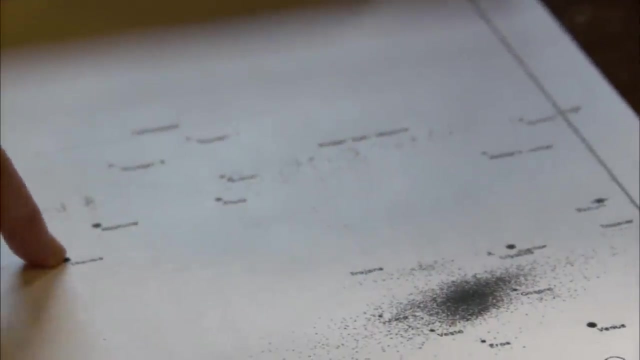 And then we see the Sun, Mercury and Venus, Mercury and Venus going around the Sun. This is the asteroid belt Jupiter and Saturn here. And here we have Uranus, Neptune and Pluto. This is Halley's Comet, which is currently out here. 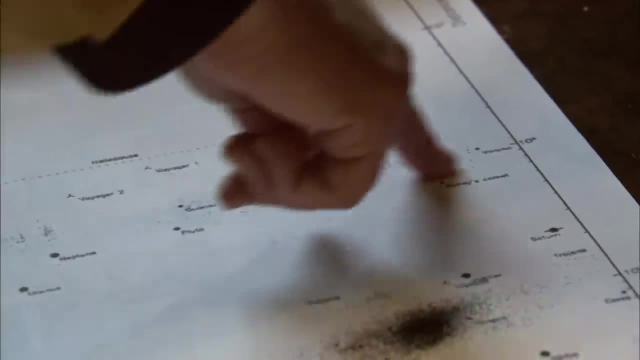 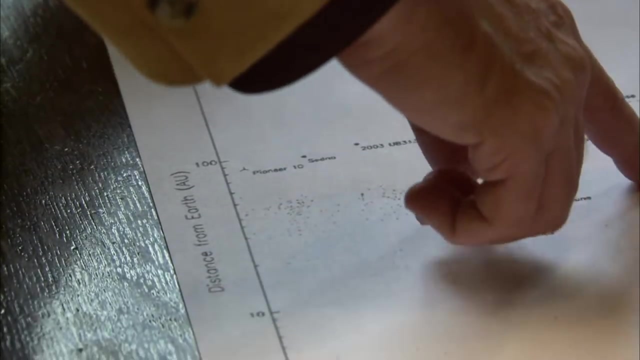 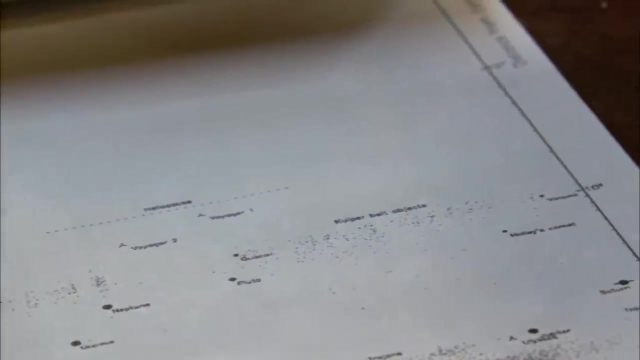 And these are the Kuiper belt objects here. These are about 700 of these that we've discovered, And these are icy bodies like Pluto. Like Pluto, Yes. And here's our spacecraft, Voyager 1 and 2 and Pioneer 10, on the way out of the solar system here. 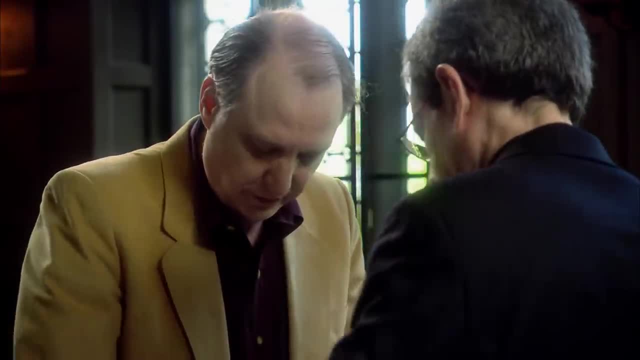 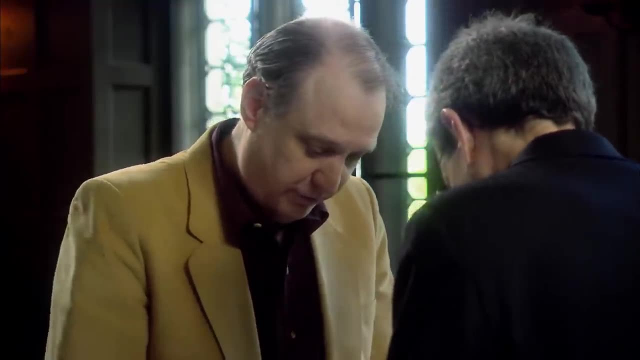 This is the heliopause, which is the interstellar medium, starts here. This is where the solar winds are And sort of ends The Oort cloud. The Oort cloud- This is where all the comets come from. There's lots of comets in the Oort cloud. 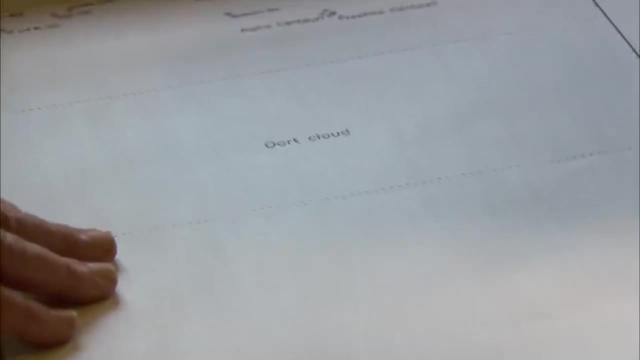 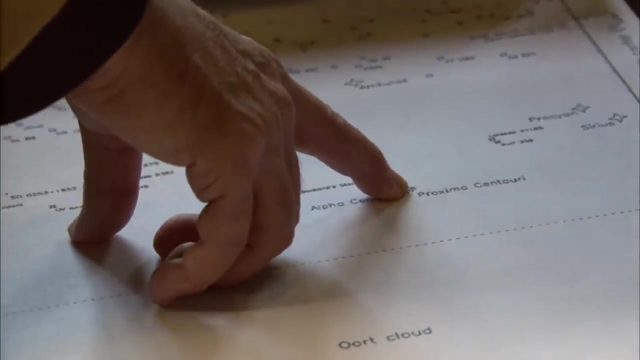 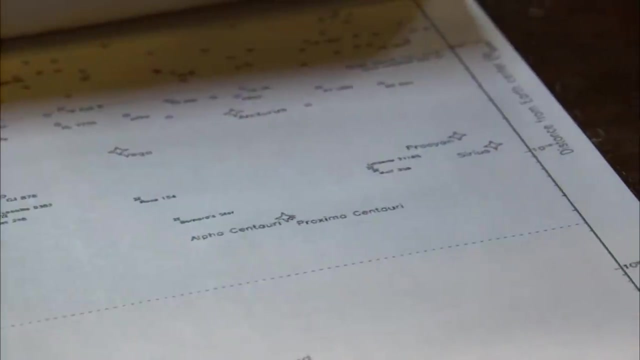 And these are periodically knocked loose into the inner solar system. This is Alpha Centauri and Proxima Centauri. Proxima Centauri is the nearest star to us, Four light years away, About four light years away. This is Sirius, which you can see in the northern sky. 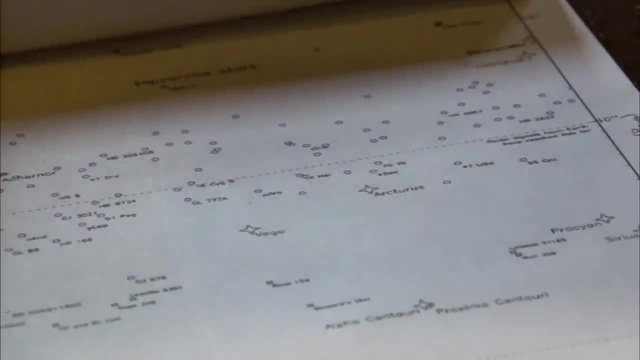 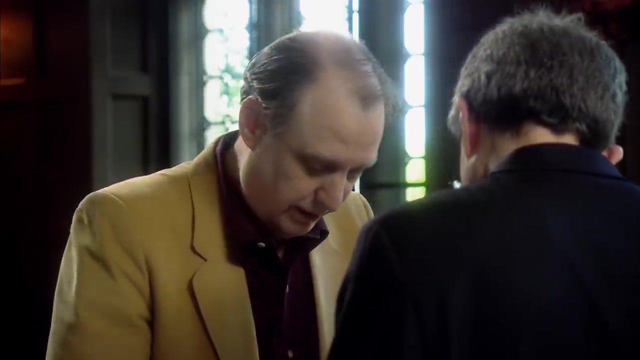 And Vega. These are quite prominent stars. And then we have here these stars that are circled, are ones that we've actually discovered planets going around. This is Cygnus X-1.. It's a black hole. This is the center of the Milky Way. 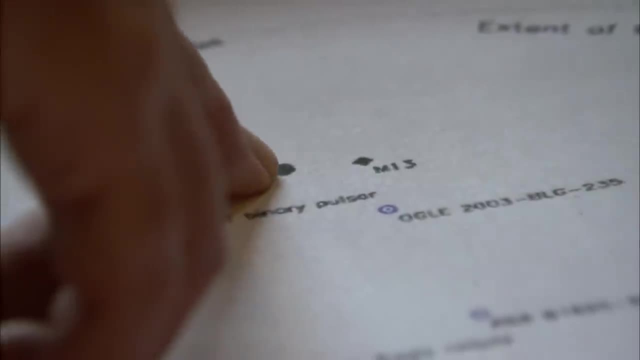 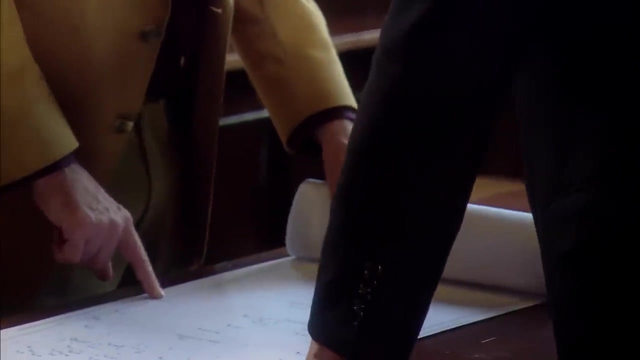 This has a black hole in it. that's about 2.6 million solar masses. There's the Crab Nebula. This is a supernova remnant that was seen by the Chinese about a thousand years ago. All in our own galaxy. This is all in our own galaxy. 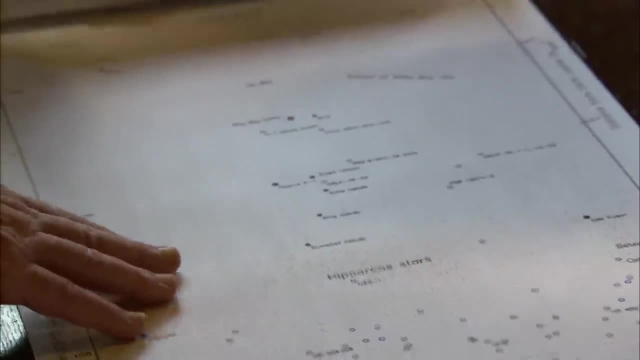 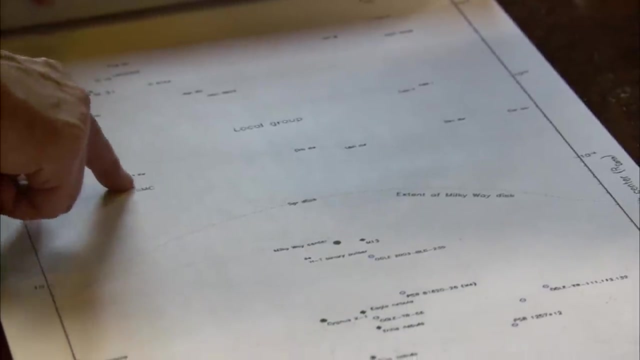 Here's the extent of the Milky Way here. This is all in our own galaxy And again, each of these is a factor of ten And further we come up here. here's the large and small Magellanic clouds. These are satellite galaxies to our own. 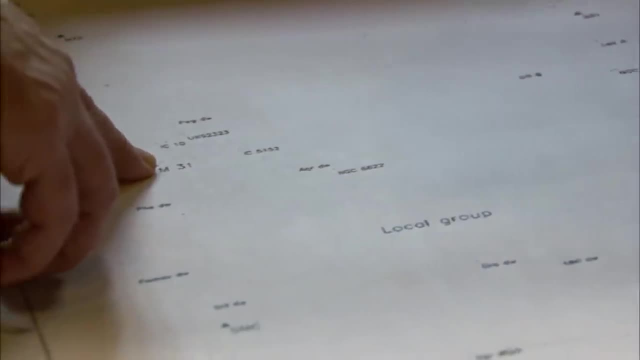 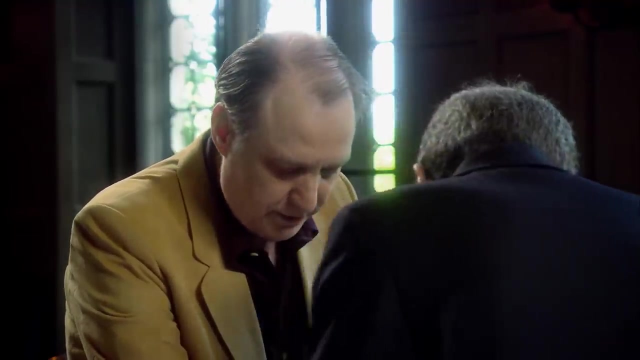 And this is M31.. This is the Andromeda Galaxy, which is the other large galaxy in the local group of galaxies. This is M87.. This is in this galaxy. in the center of this galaxy, We've discovered the largest black hole. 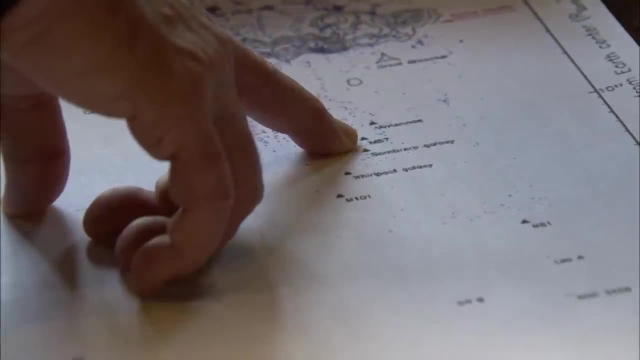 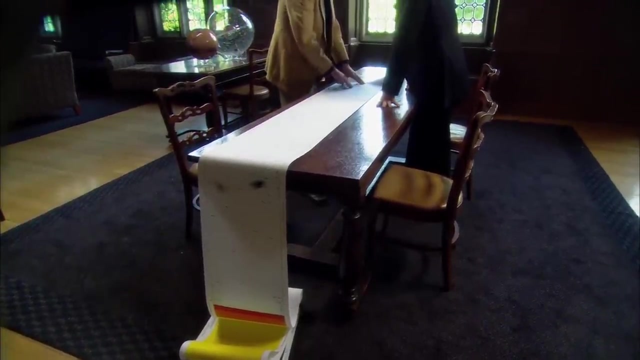 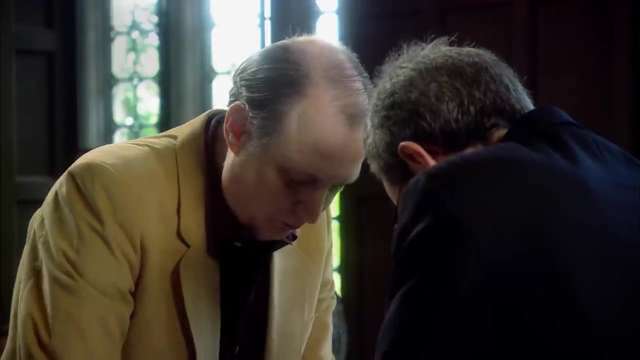 This is a 3 billion solar mass black hole in the center of this galaxy. And then we start to get galaxies. here in the Sloan Survey We have 125,000 galaxies that we've plotted And we see a lot of structure. Here's the voids, here. 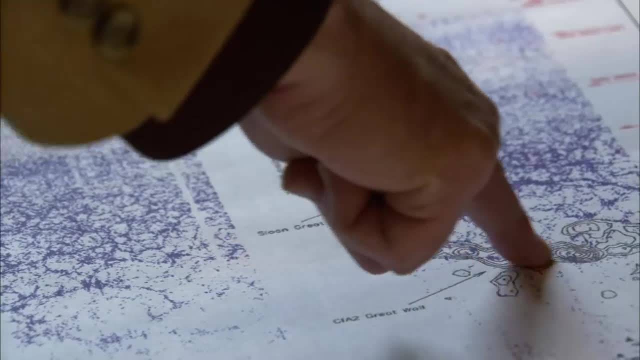 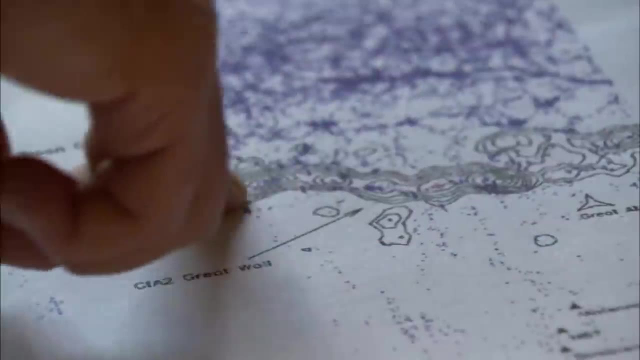 And we start discovering great walls of galaxies. This is a great wall of galaxies discovered by Geller and Hooker called the Great Wall. It's about 750 million. It's about 750 million light years long And this is a Sloan Great Wall, which is in the Sloan Survey. 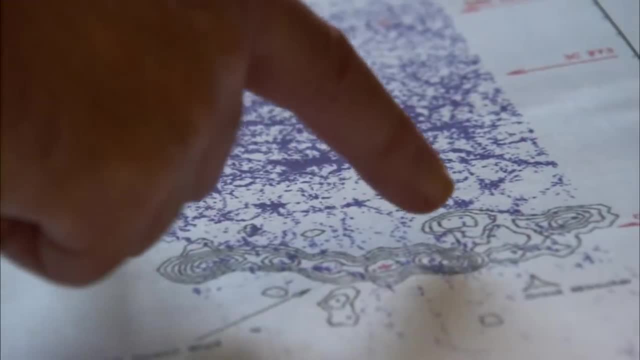 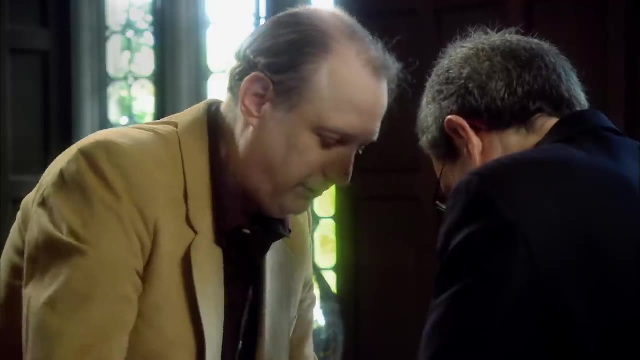 This looks like two-thirds the size, But actually it's three times further away. It's 1.37 billion light years long. It's the largest structure that we've found in the universe. How many galaxies would be in this Sloan Great Wall? 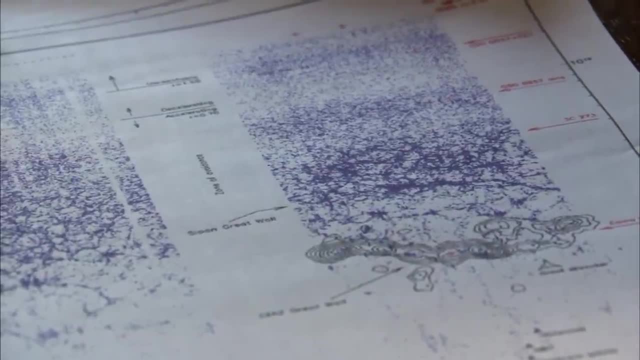 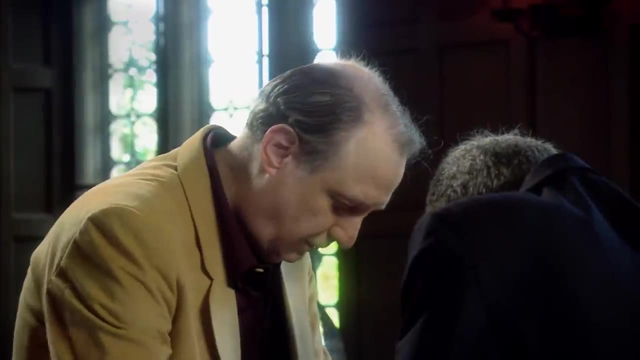 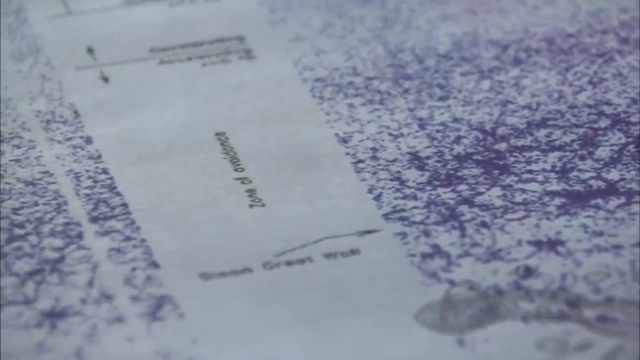 There's about 10,000 here in this And it has many rich clusters and groups of galaxies And it's an extraordinary structure And you'll notice that there's a sort of sponge-like structure here of these great walls, And this is something that you'd predict from inflation. 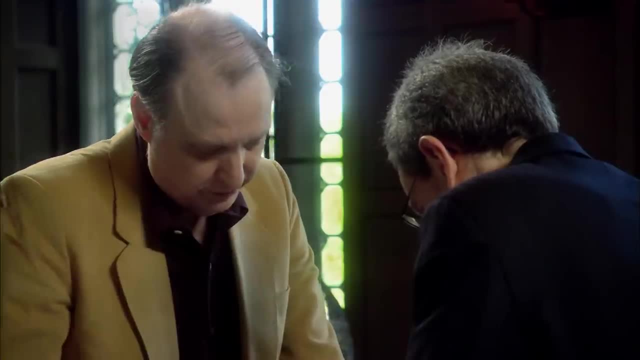 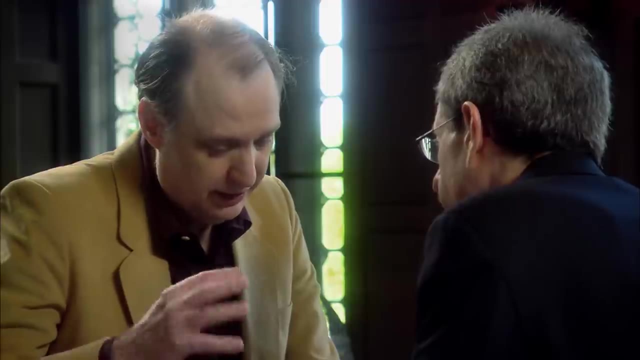 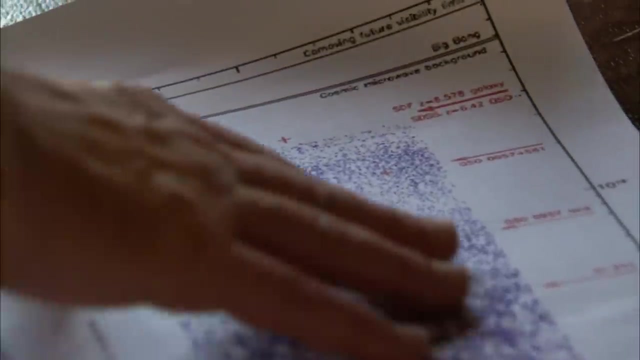 Inflation predicts that these structures are due originally to small, random quantum fluctuations. And if these are random, you expect the high-density and low-density regions to look the same, And a sponge does that. The insides and outsides of the sponge are the same. 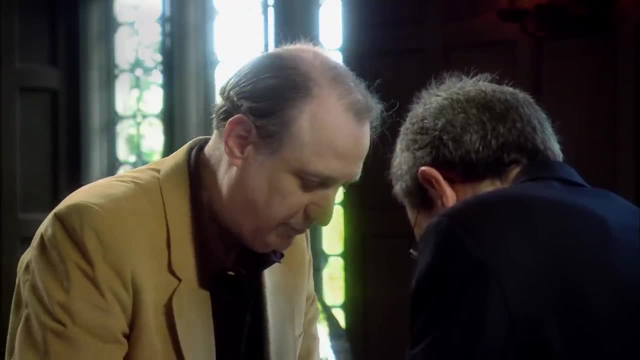 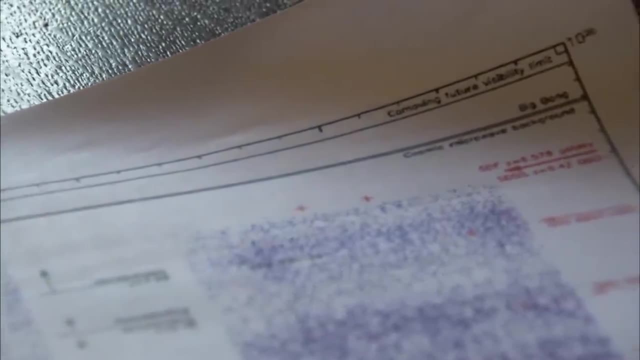 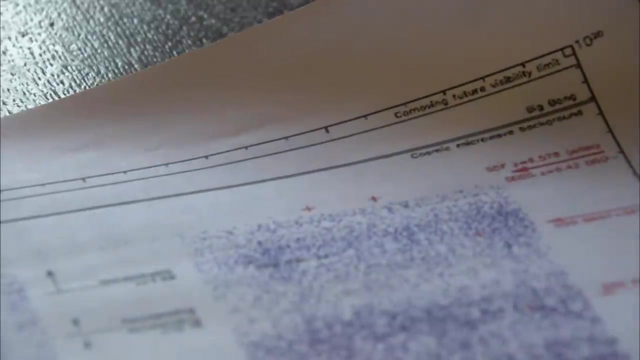 So we have this complicated sponge-like pattern of galaxy clustering here, And then, finally, here's the cosmic microwave background. It's the furthest thing that we can see. It's light coming to us, radio waves coming to us from when the universe was only 380,000 years old. 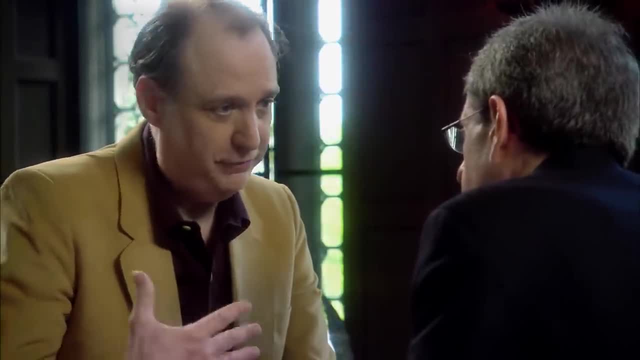 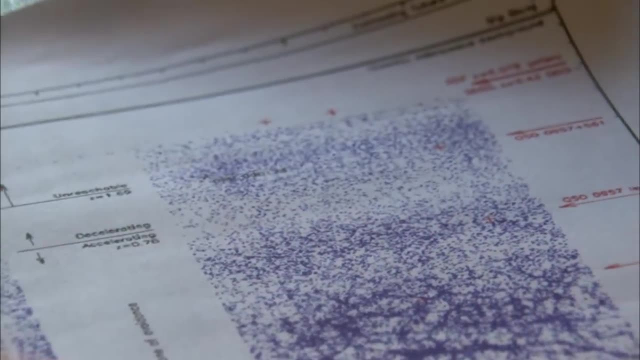 Because before then it was opaque. Yes, it's like a fog. You're looking into a fog bank, So it's the furthest that you can see, And this is about 13.7 billion light years away. That's how old the universe is. 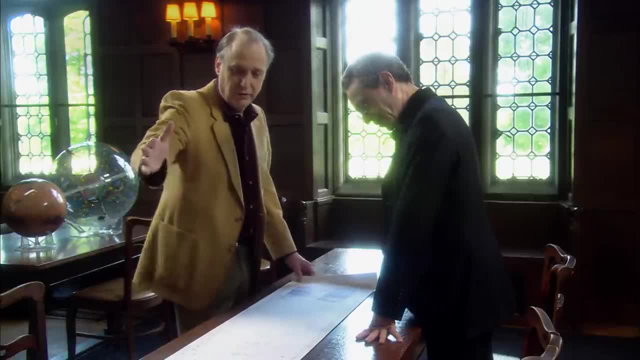 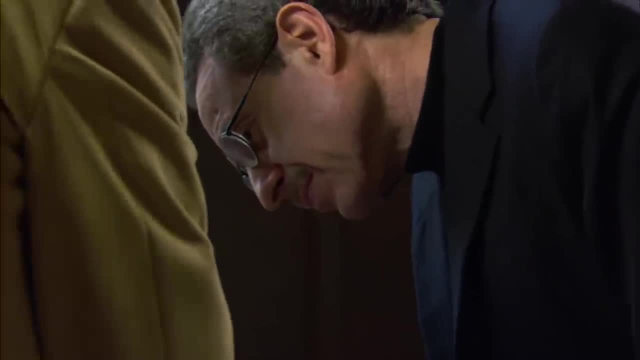 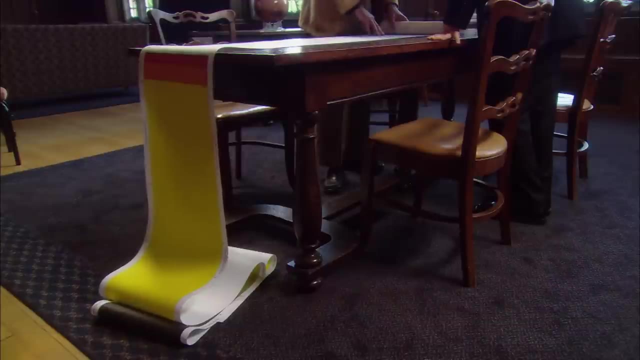 That's how long it's been coming from us. That's very exciting. This is the whole universe on one map. Wow, Riveting. What more to say? The entire universe rolled out on one sheet of paper? Yes, a long one. 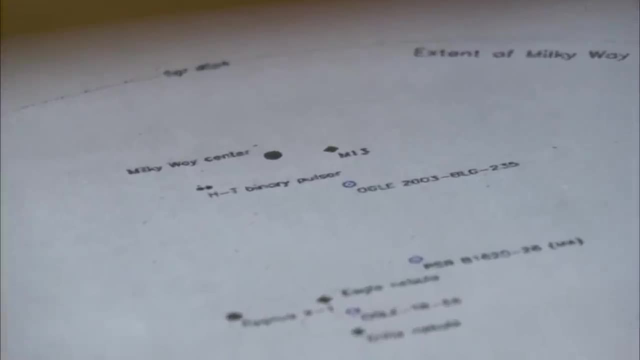 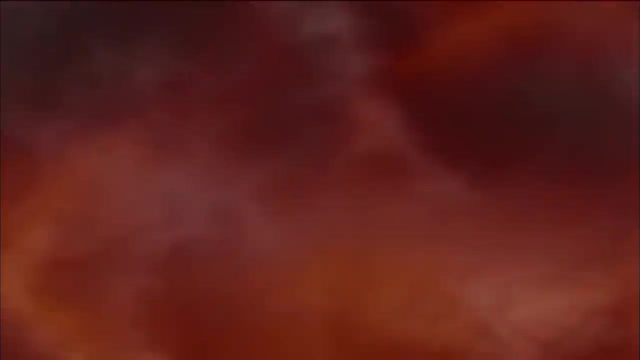 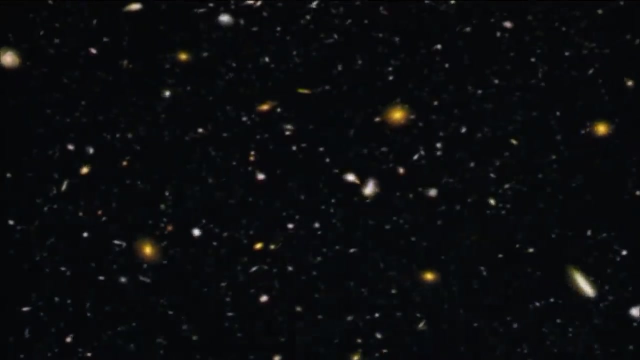 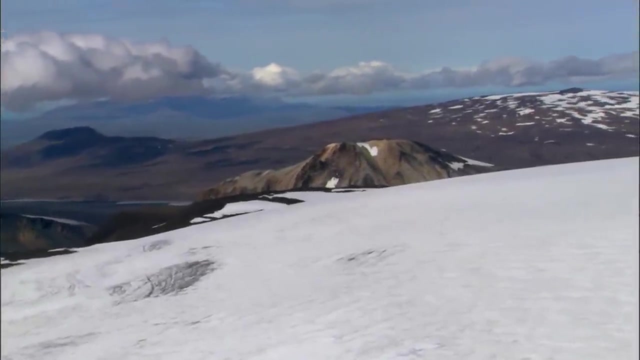 How could such wondrous complexity arise? Billions of galaxies, all originating from a sizzling soup of furiously hot plasma, emerging out of the Big Bang and expanding outwards. I go to Iceland for a meeting of the Foundational Questions Institute. 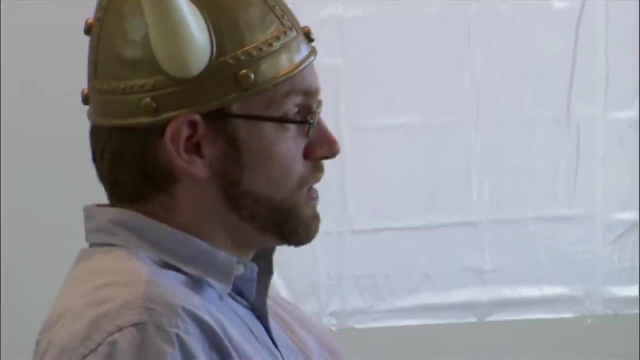 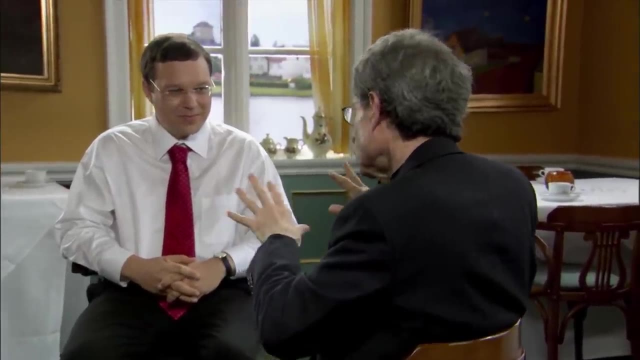 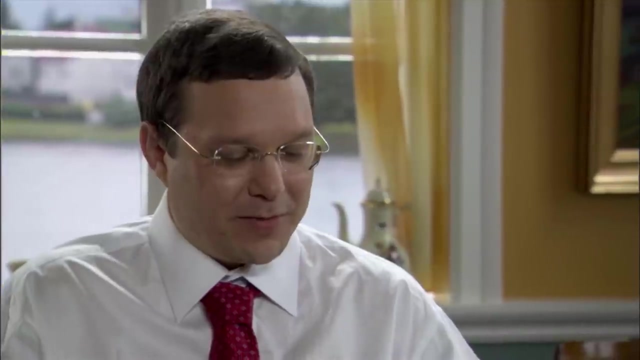 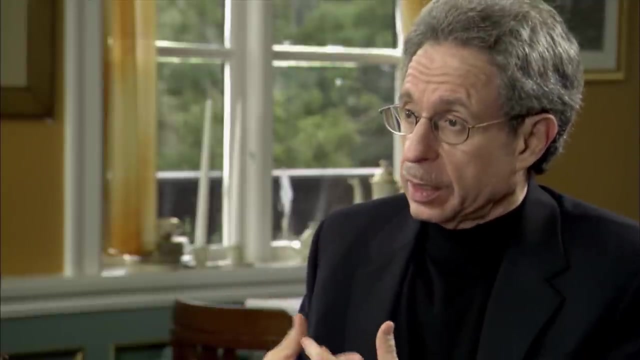 FQXI, where physicists and cosmologists dare to dream. I meet astronomer Avi Loeb, originally from Israel, now at Harvard. Avi's an expert on how galaxies formed and evolved. I ask him how we got from the Big Bang soup. 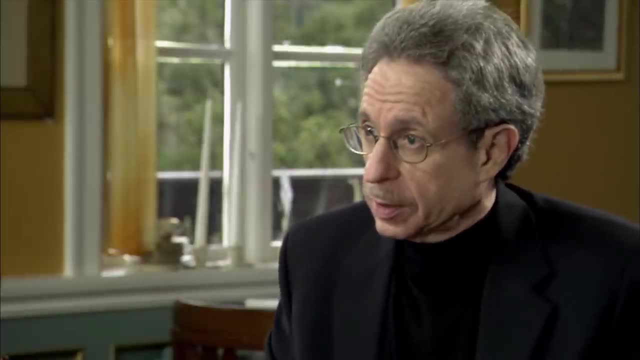 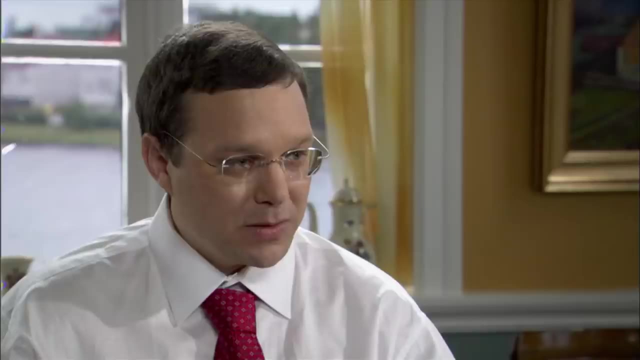 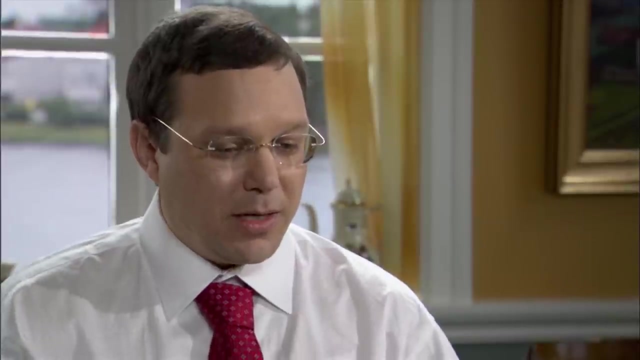 to the galactic structure we see today. The simple answer to that is gravity. What gravity did is start from these initial conditions and make the universe much more complex. How did it do that? There were density fluctuations in the universe. The density was uniform by and large. but there were small fluctuations, small differences in density from region to region And if you consider a region that was slightly more dense than the mean density of the universe, this region acted upon itself by its own gravity and made itself even more dense with time. 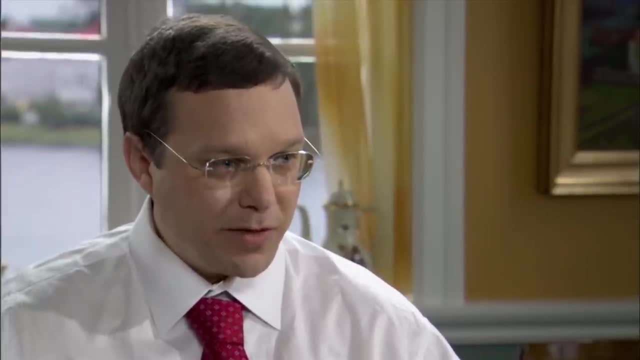 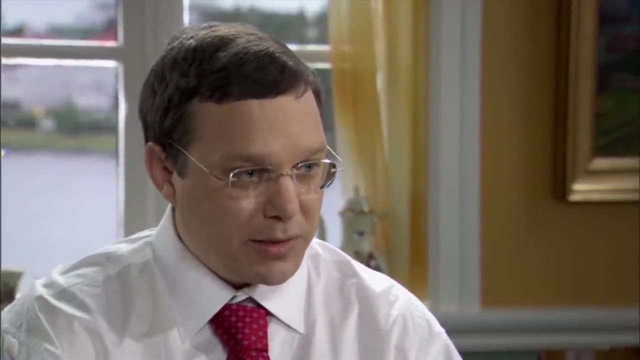 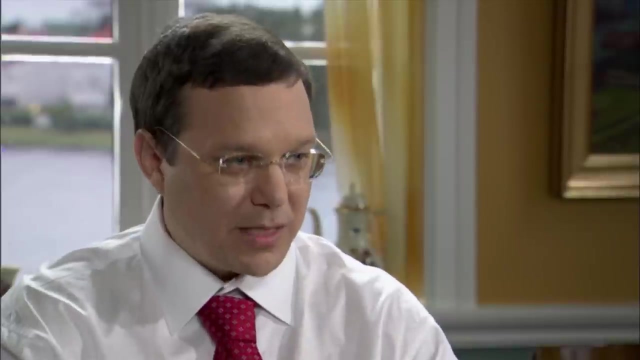 So, in fact, instead of expanding with the rest of the universe forever, it drew matter into this region so that eventually, the region collapsed upon itself and did not participate in the cosmic expansion. And that's how an object was made out of such a region. 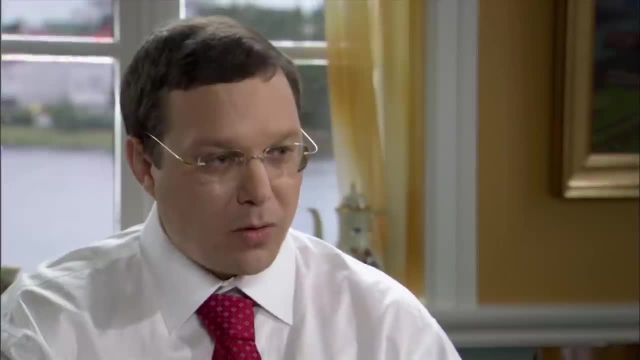 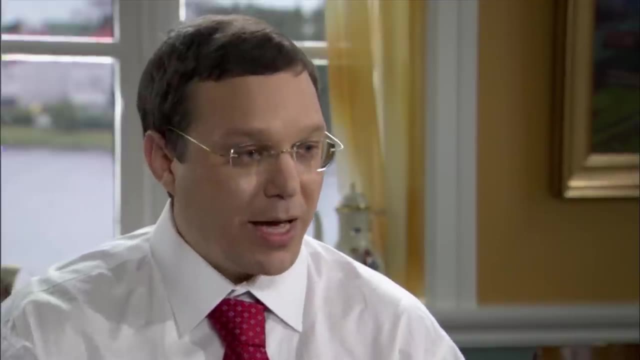 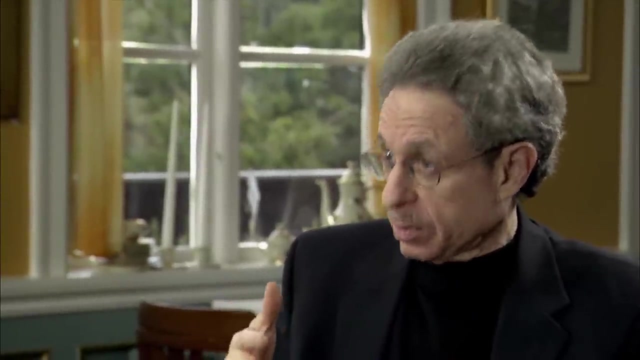 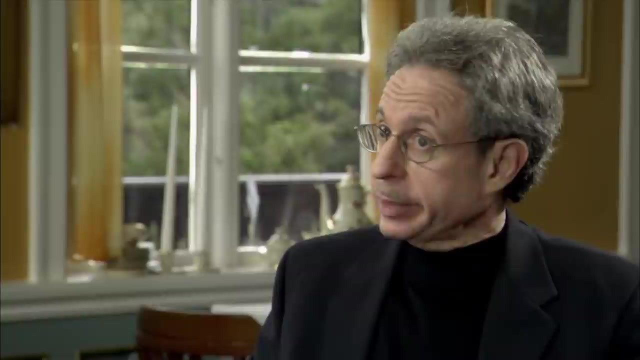 And the universe was filled with small density and homogeneities that resulted from inflation due to fluctuations, quantum mechanical fluctuations. So it's these inhomogeneities, these small fluctuations caused by quantum fluctuations, that later emerged through gravity over time into the structures that we see in the universe. That's correct. These were the seeds that were implanted by inflation that later grew to become the objects that we see nowadays, just like the seeds of a tree that are smaller than the tree itself. And they were small and gravity made them bigger with time. 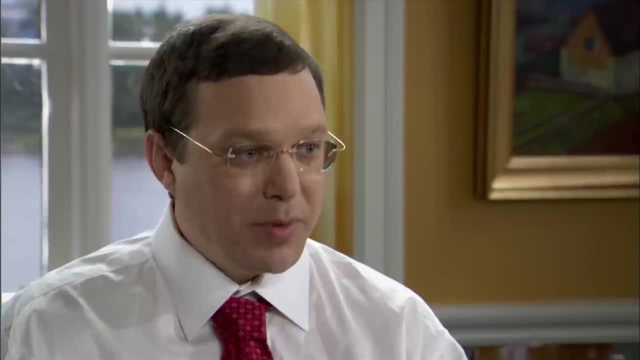 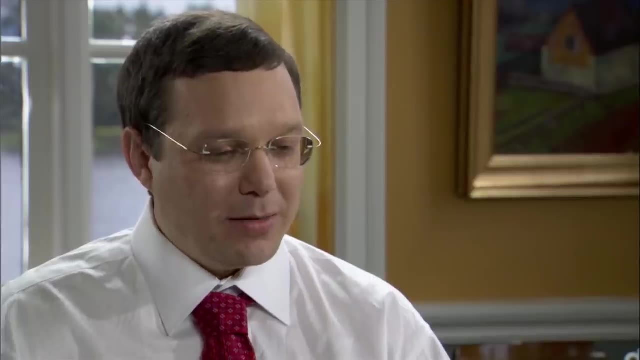 Now you may ask: when did the first objects appear in the universe? So inflation ended around 10 to the minus 35 seconds, And after that there was a long period of time during which radiation was the dominant constituent in the universe. 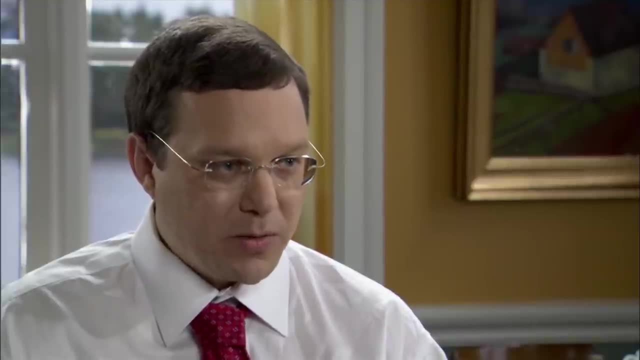 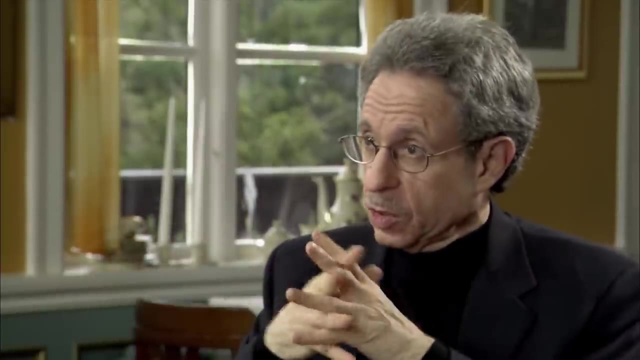 And during that time no objects could be made because the radiation would suppress the formation of objects, And it was very opaque. You couldn't see anything because the radiation was just bouncing off. everything That's correct. And then, about 400,000 years after the Big Bang, 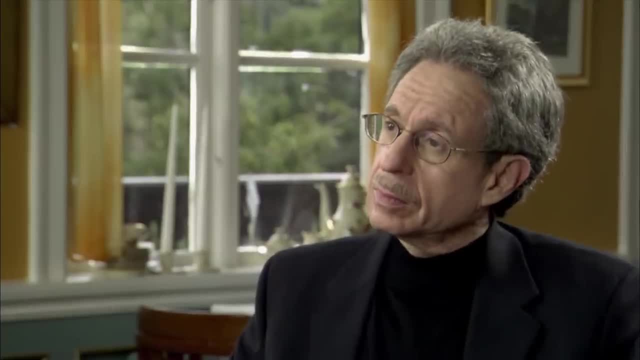 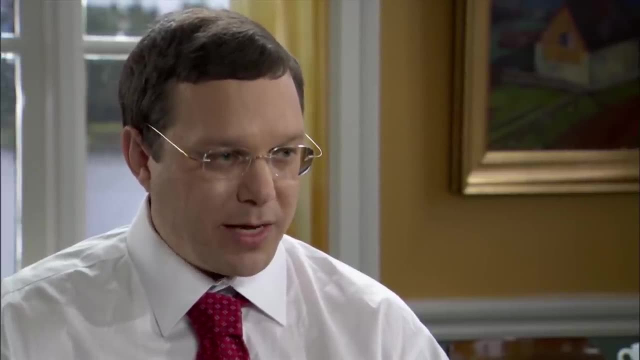 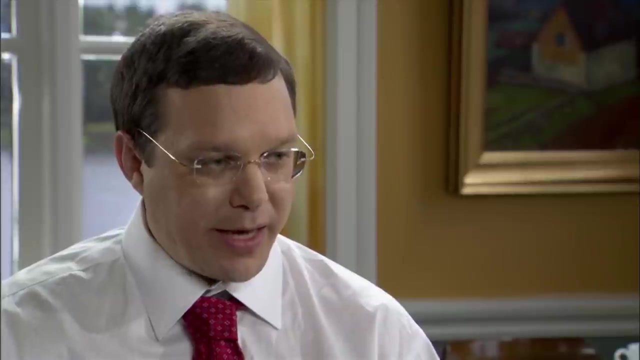 the gas. due to the cosmic expansion, the gas was able to cool to a point where hydrogen atoms formed out of it, And because of that the radiation was able to stream freely through the gas and decouple from it, And then the gas was able to condense into objects. after that, 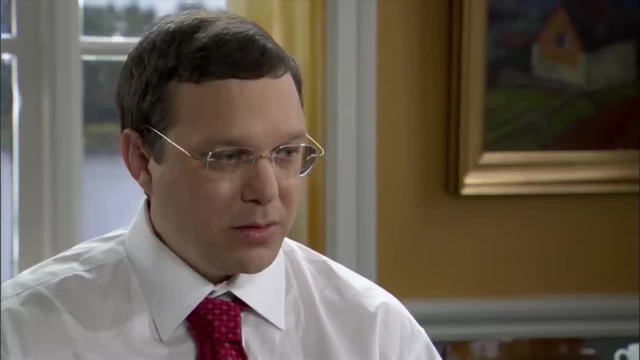 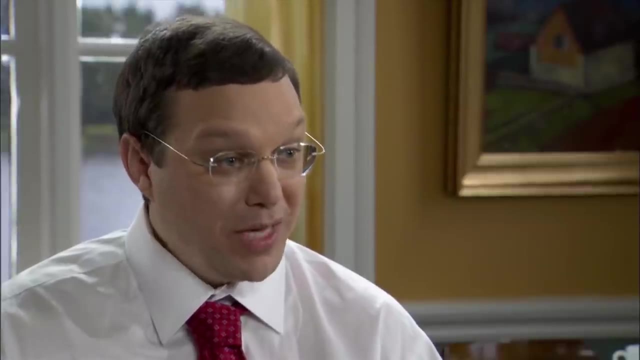 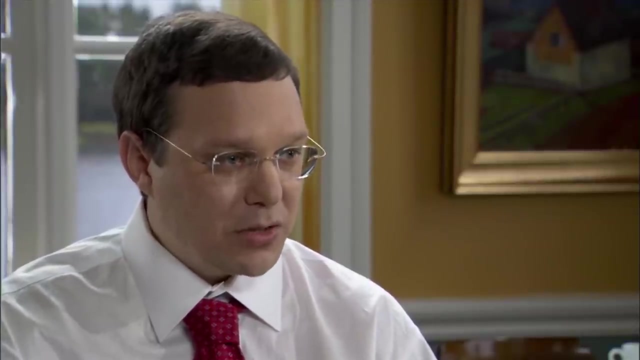 And it took some time before the first objects appeared. According to theory, the first objects appeared when the universe was about 100 million years old, And then the first stars formed inside these condensations And they produced radiation that, in principle, we can see. Now from that first object. how long did it take to have the first star? Because you needed a critical mass so that it would implode on itself and you'd have enough heat and pressure to cause fusion reactions among hydrogen to create the thermonuclear activity. That process was very quick, About a million years, And as time went on, because of the unstable nature of gravity, the small inhomogeneities grew and became, eventually collapsed into making objects. They first collapsed into sheets And when the sheets intersected, 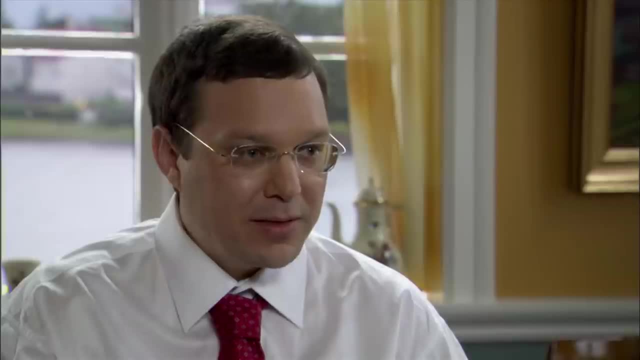 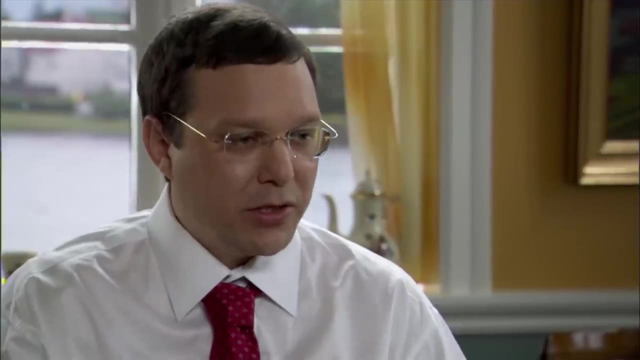 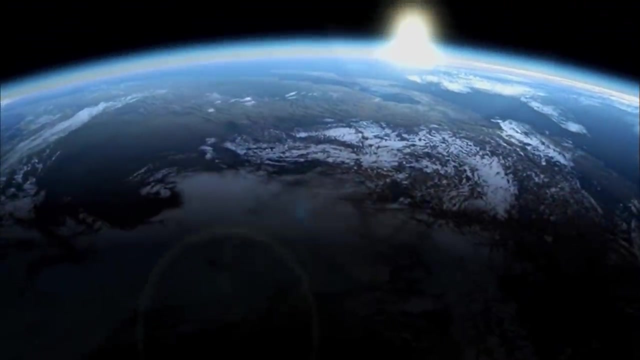 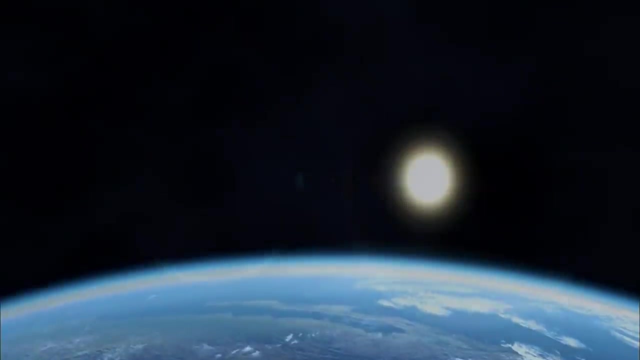 they made filaments, And then material from the filaments was channeled into the intersection of the filaments and made galaxies and eventually groups of galaxies, Gravity operating alone, slowly but inexorably, working its wonders, coalescing innumerable atoms. 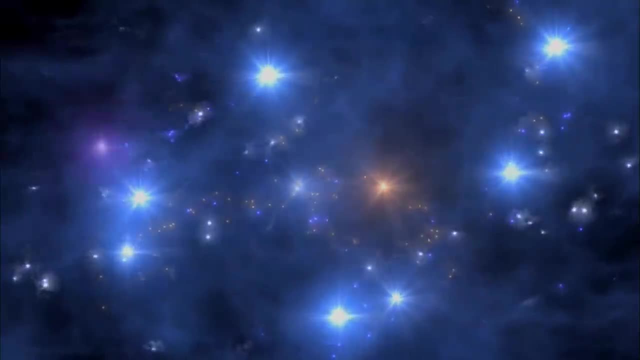 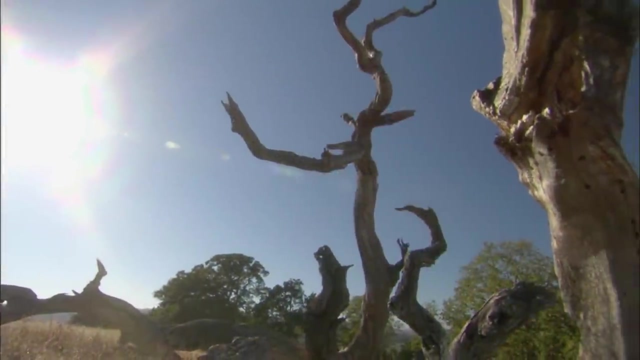 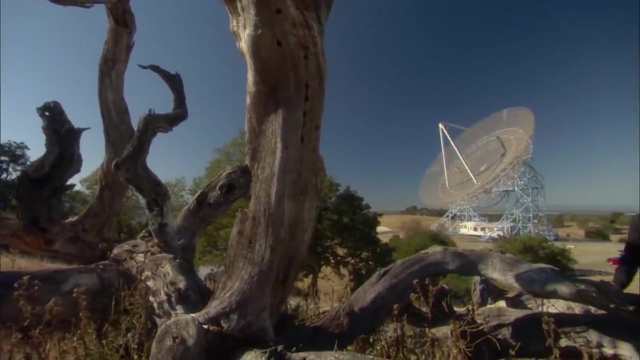 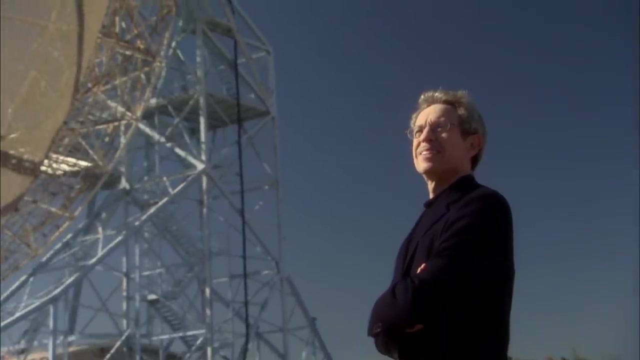 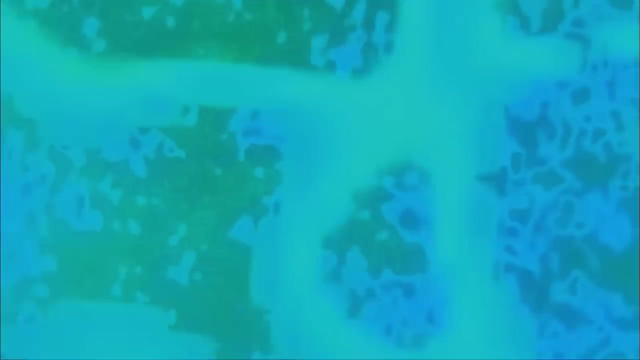 floating and flowing randomly into the magnificent large-scale structure we see today. It seems incredible that something so simple- gravity- can generate something so complex- Life. But is this just a story? Is there any real evidence I'm told about a baby picture. 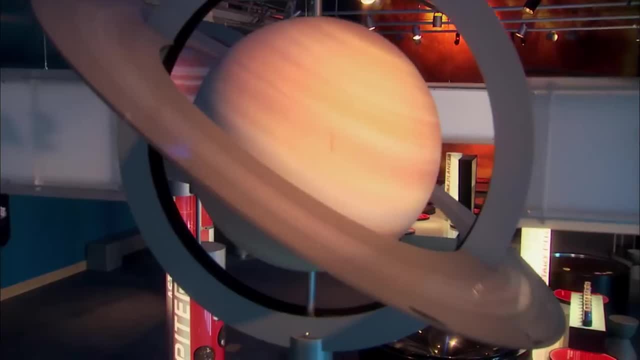 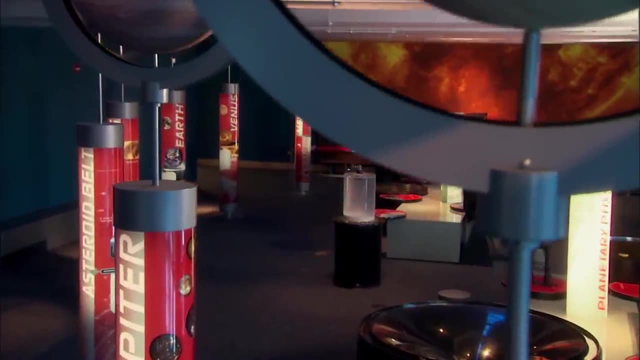 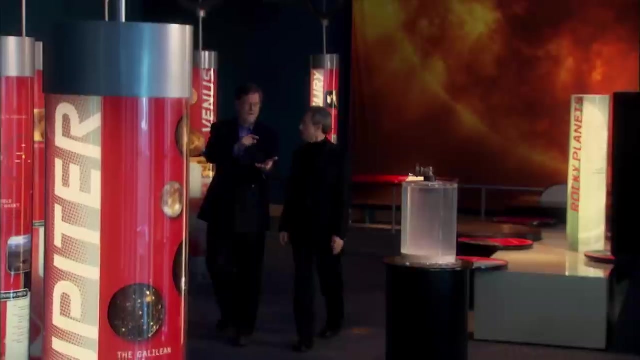 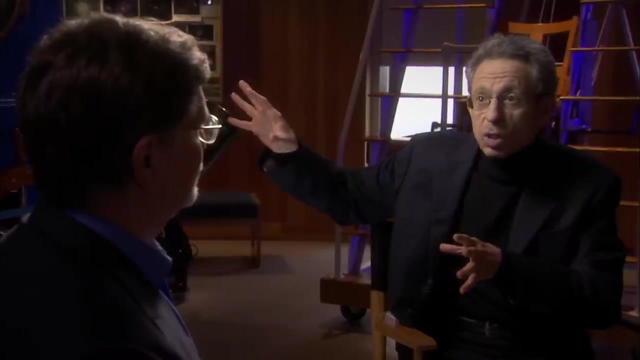 of the early universe. I go to Berkeley to meet the man responsible, George Smoot. For taking that picture won the Nobel Prize. George, what is the picture of the early universe that can give hints of what these huge structures would become? 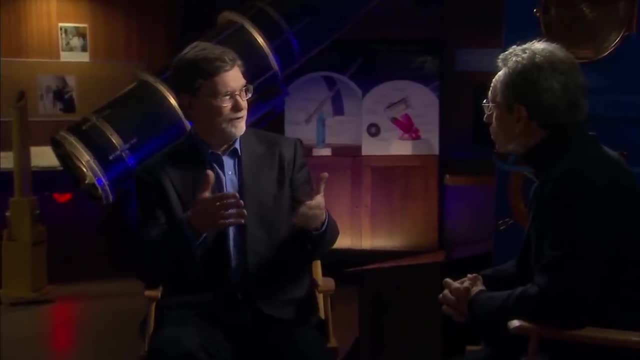 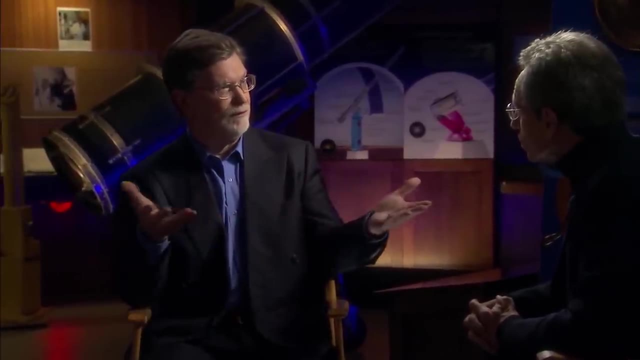 So with the cosmic microwave background we make the picture of the embryo universe, And what it shows us is the universe itself is extremely homogeneous and expanding very uniformly in all directions, But there are all these small variations at the part in 10,000 level. 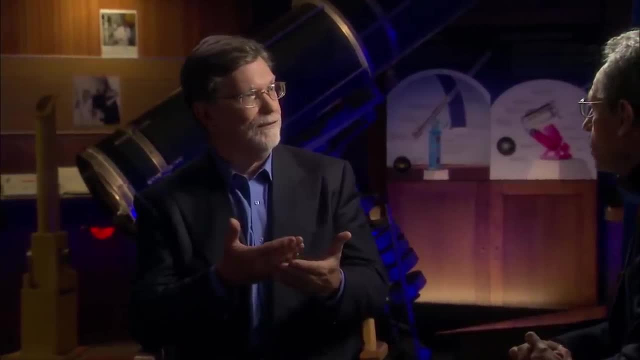 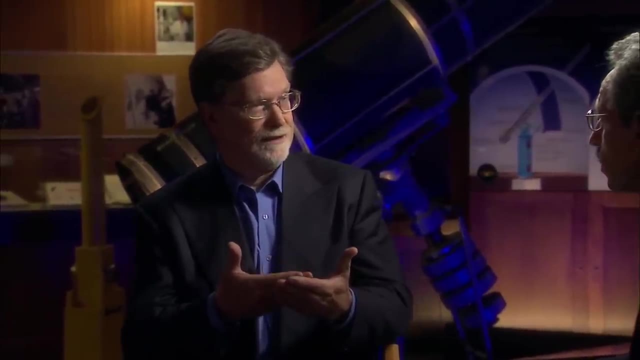 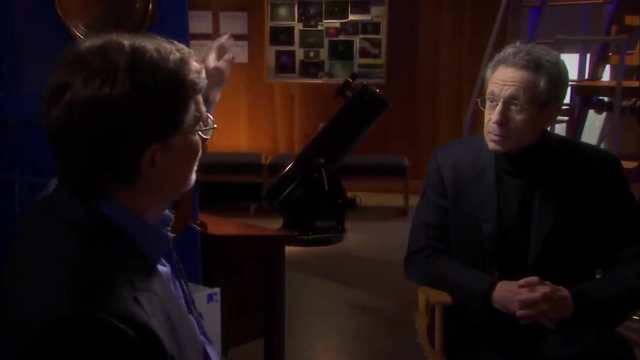 and those variations are there present, with average variation equal in all scales. It's completely scale-invariant at the beginning. That is, if I look on the scale of the horizon as far as I can see in all directions, I see a large-scale variation across that. 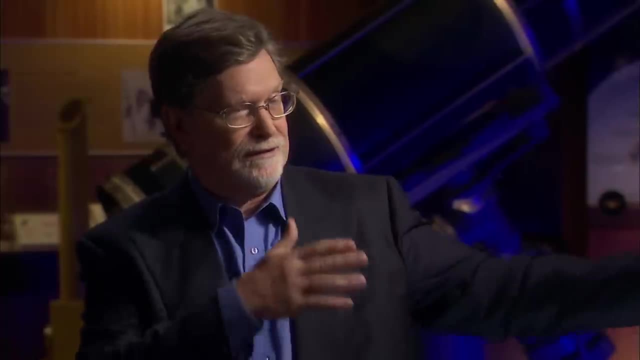 and its average variation is about a part in 10,000.. And if I look, say, a third of the way across the horizon, I see the same sort of variations, just random fluctuations. And if I look down to tiny scales, 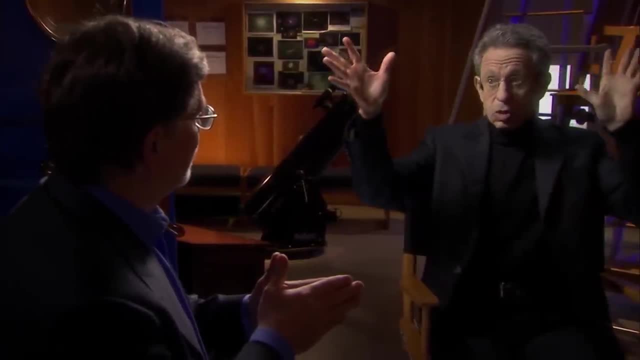 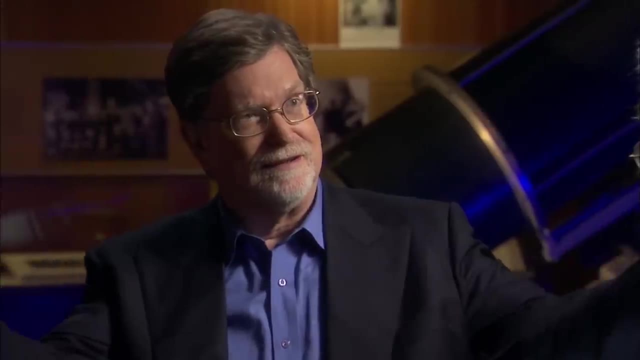 I see the same thing, And so, And this is across the whole sky, This is across the whole sky When you do the cosmic microwave background radiation, it's everywhere And what we're basically seeing is, you know, looking out and seeing the surface of a sphere. 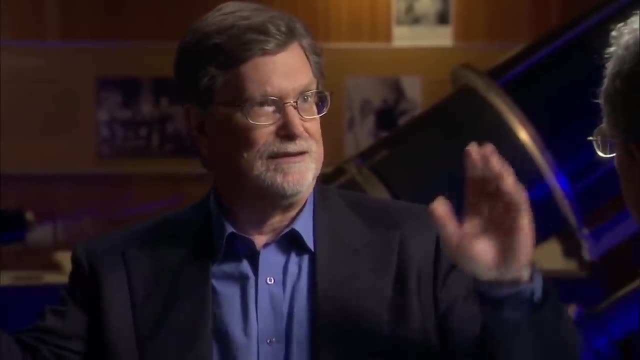 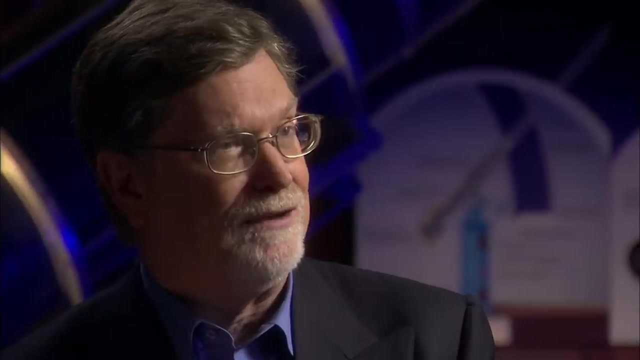 that's 14 billion light-years away from us, and we can imagine that any samples of surface of spheres have roughly the same appearance. It's just random variations that we see stars in, And so we can make up this map. we can do computer simulations. 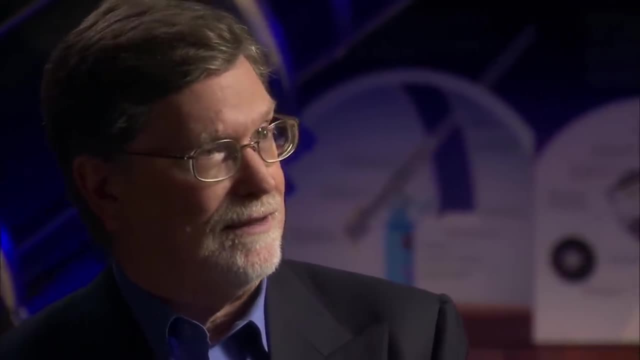 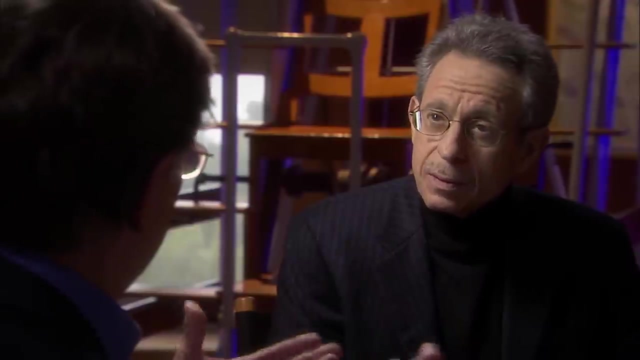 and we see this evolution And the thing that has happened is the things that are really big. the matter hasn't had time to move around, so they're pretty much primordial and they haven't formed their large-scale structure. But when you get down to the scale size of the Great Wall, 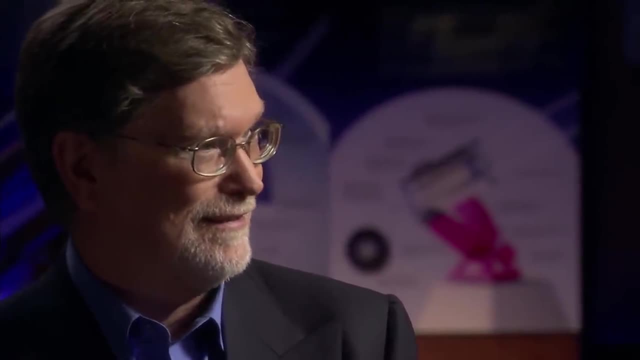 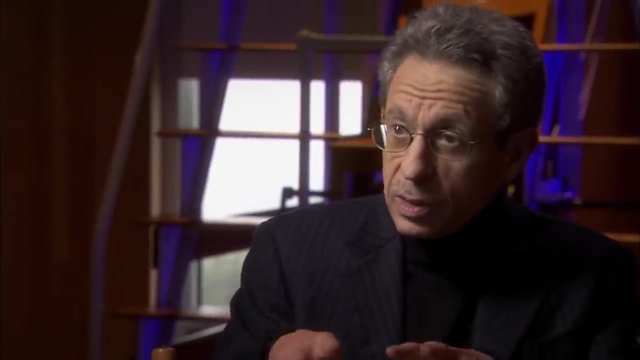 and then you know clusters of clusters of galaxies. they're the biggest things that will form, because now we shut off the formation of structure by the accelerating expansion of the universe. But what's particularly remarkable is that you can forecast all of this Right. 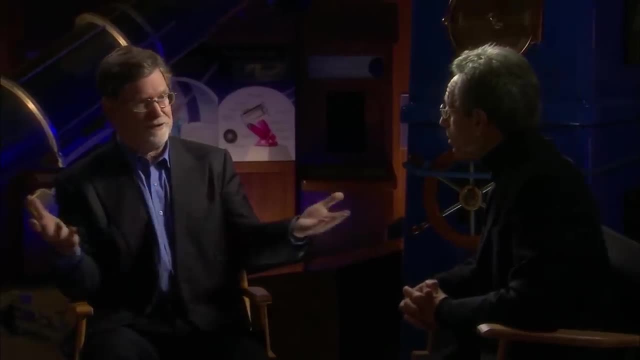 from the picture of the early universe. That's right. You can start with this very simple case. basically a homogeneous soup. It's like a glass of water with just a few specks in it and those are going to grow kind of like mold. 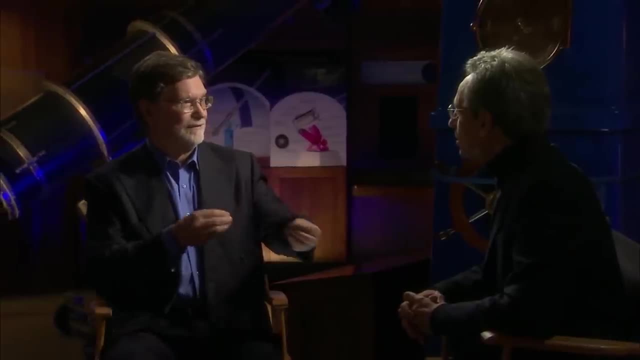 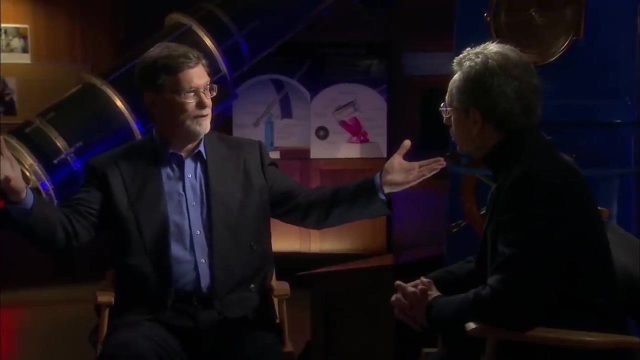 except it's by gravitational absorption. You can do those calculations. You just need Newtonian gravity or Einstein gravity. It's simple, But you just start and you just let 14 billion years go by and gravity pulling it in and eventually you'll find this: 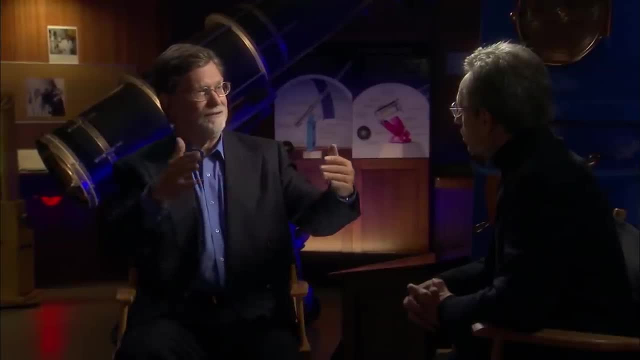 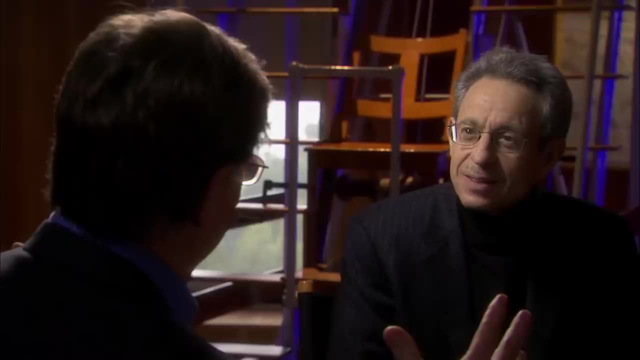 what we call the cosmic web, this structure where there are these large like dirty cobwebs of galaxies. You know they're beautiful, They're nice shining lights in the sky that are just. you know, take your breath away when you look at it. 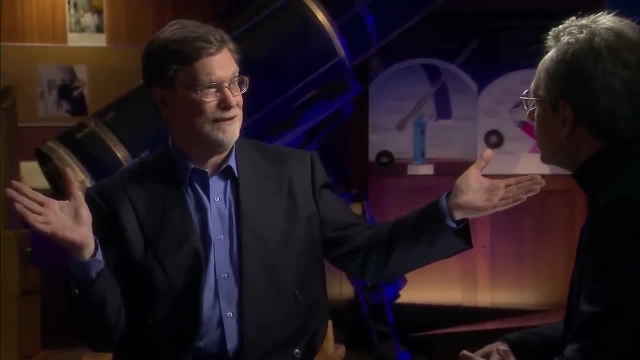 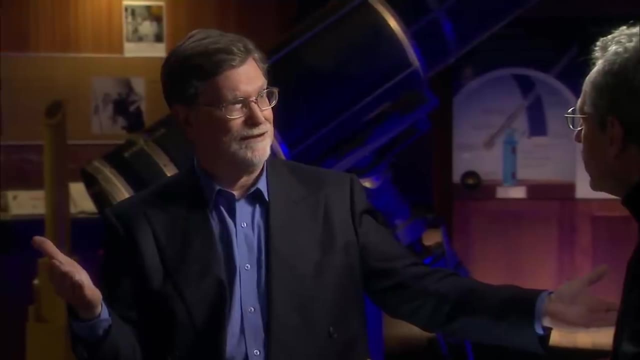 So you know, I look at that picture and I see millions of galaxies in that picture and I go, you know, wow, Every one of those was a quantum fluctuation and it just got expanded by the expansion of the universe to be this scale. 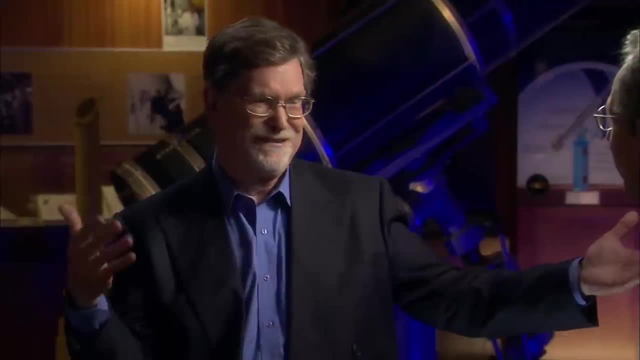 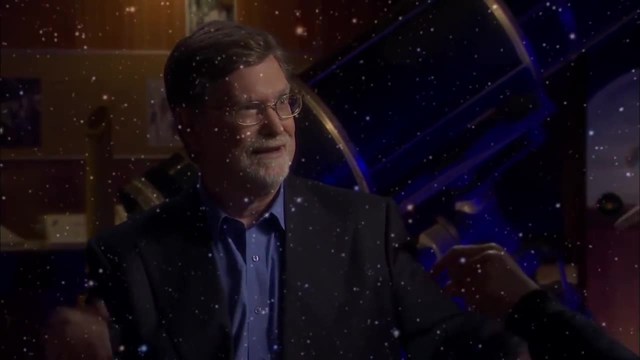 and then all you had to do was cook it for sort of let it cool on the stove, so to say, for the 14 billion years. and then you got these. you got these beautiful jewels. It's just started. We know where it is now. 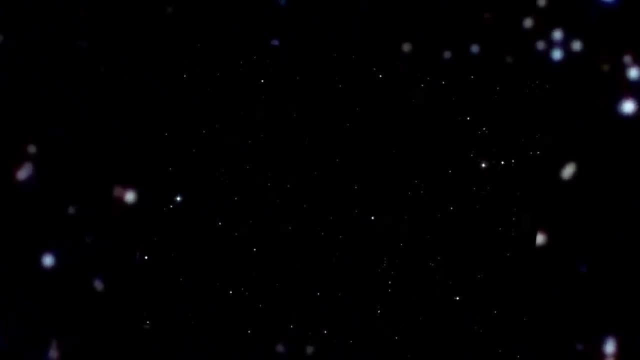 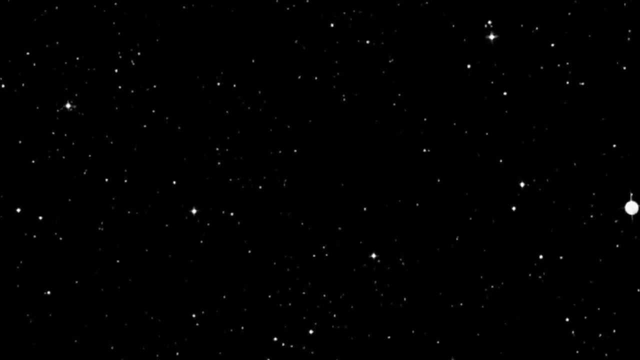 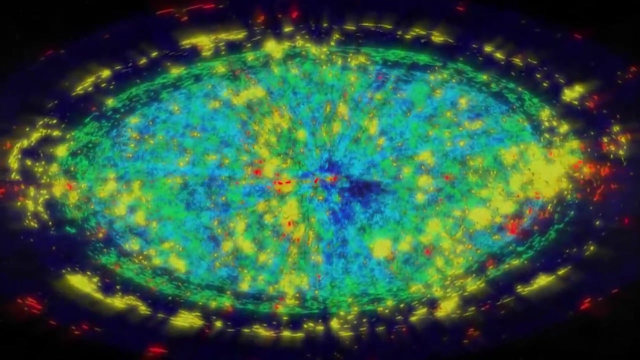 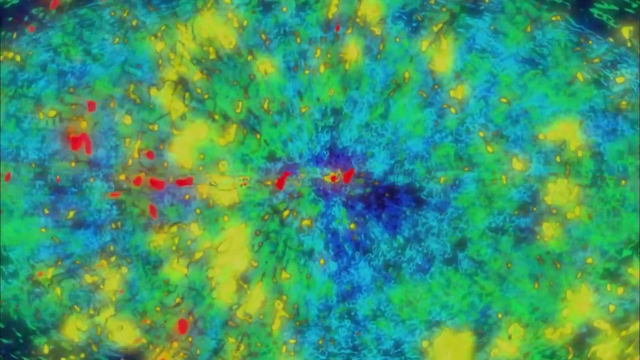 I am in awe of what we humans have discovered. Almost 14 billion years after the Big Bang, we can see, literally see, its afterglow. The Nobel Committee called observing the cosmic microwave background radiation the starting point for cosmology as a precision science. 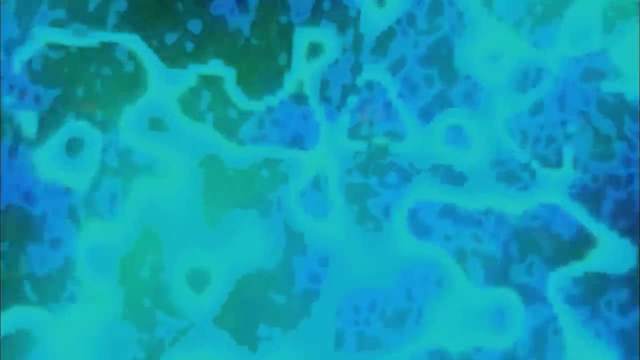 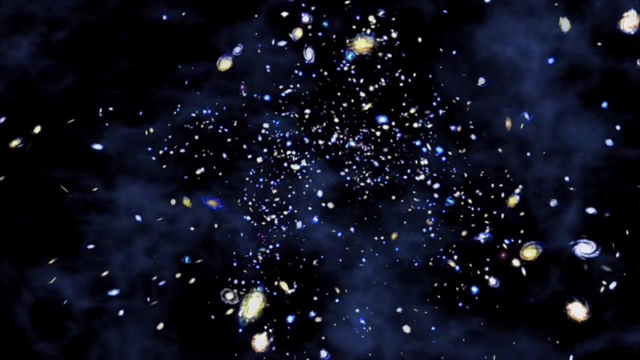 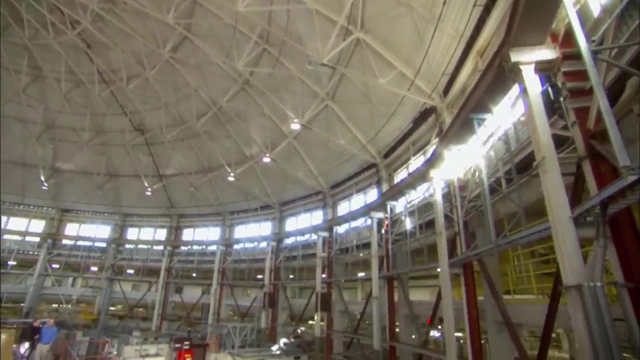 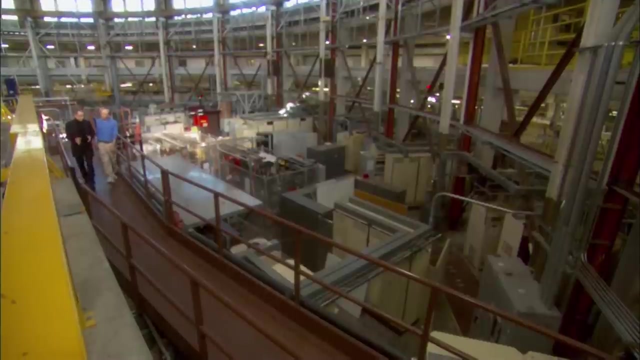 That's the real evidence for the early history of the universe. Now, what about the future of the universe, its ultimate fate? I go to Lawrence Berkeley National Laboratory to meet the man responsible for one of the biggest shocks in scientific history, Saul Perlmutter. 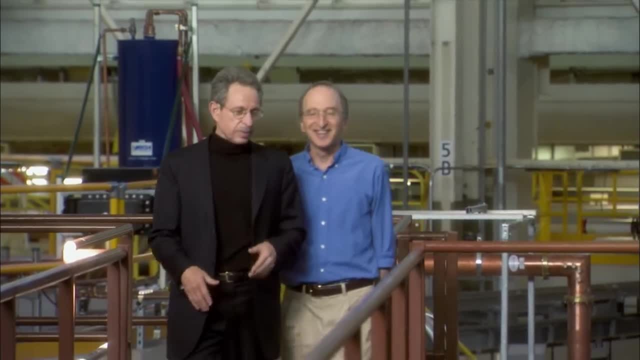 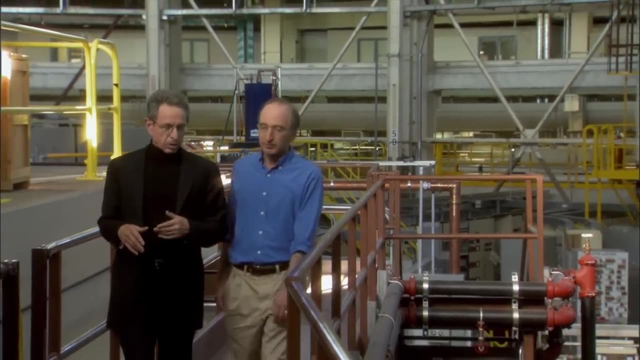 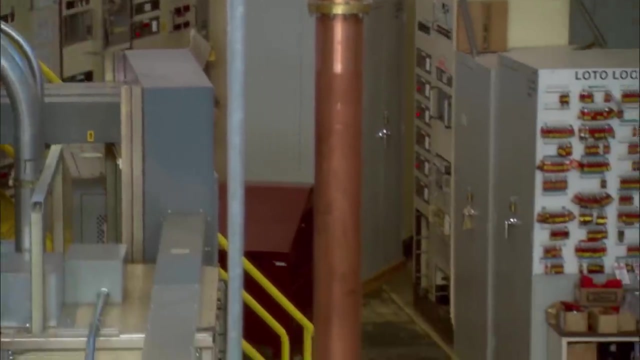 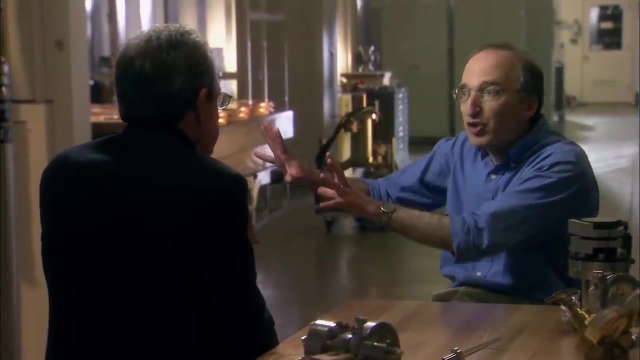 Everyone had expected that, due to gravity, the expansion of the universe would be slowing down. Saul discovered that the expansion of the universe was speeding up. I asked Saul about dark energy, the mysterious force that powers, apparently, the accelerating expansion of the universe. 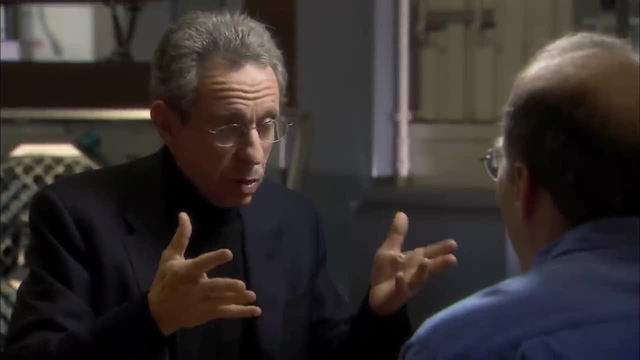 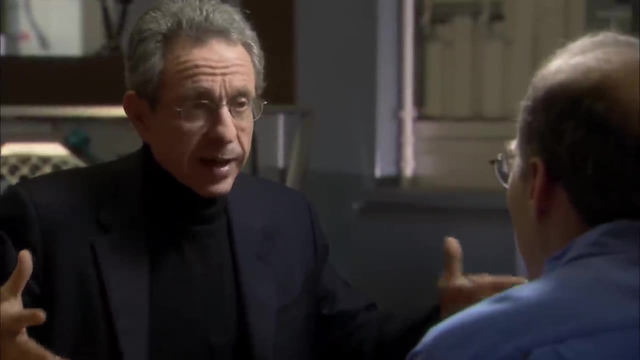 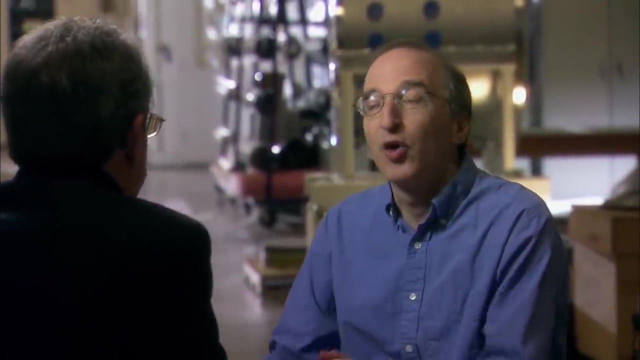 Some of the data that you've remarkably observed and developed, particularly as it affects dark energy. how does that affect this large-scale structure? It actually turns out to make a big difference because if you live in a universe where it's always slowing down in its expansion, 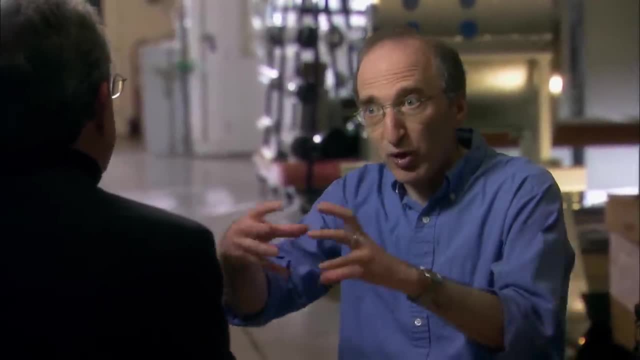 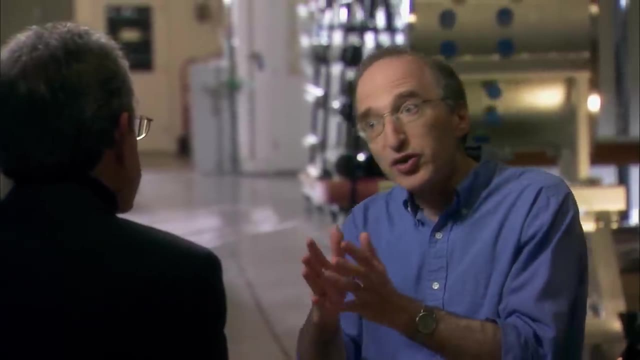 in some sense it makes it easier for you. it makes it easier to form structure because things can be attracted in and fall in towards each other more easily If you live in a universe- as apparently we do- which has started to accelerate and expand faster and faster. 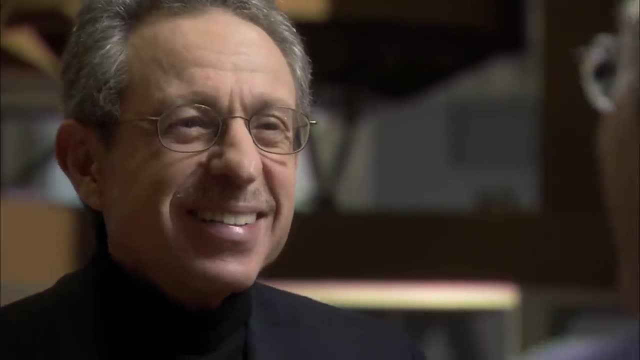 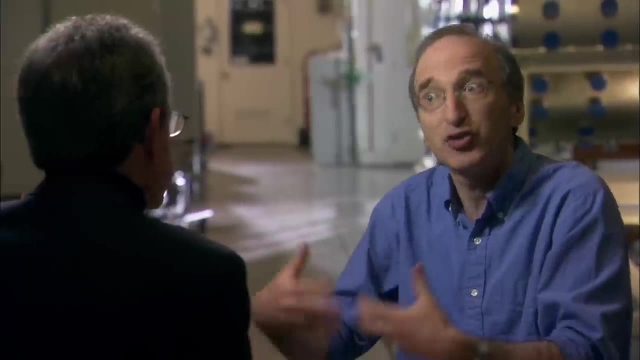 in some sense, now you're trying to, you know, run down an up-escalator. There's something that's trying to pull things apart at the same time that you're trying to congregate galaxies and clusters of galaxies, and that changes that whole picture. 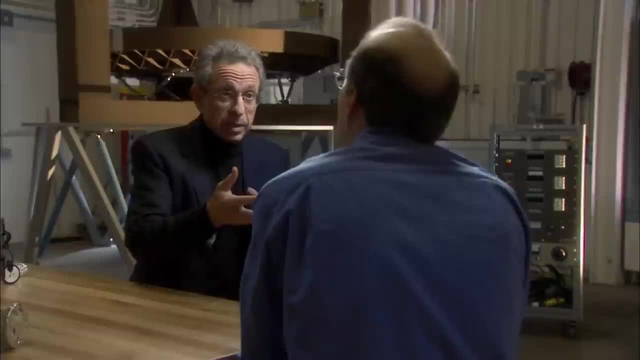 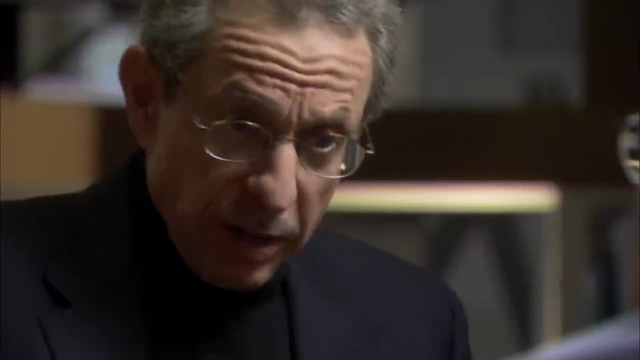 of how the structure forms. So you need dark energy, You need some extra push to make the universe get a little bigger at the very end, or you won't see what we see today. Now, is it fair to say that the dark energy? 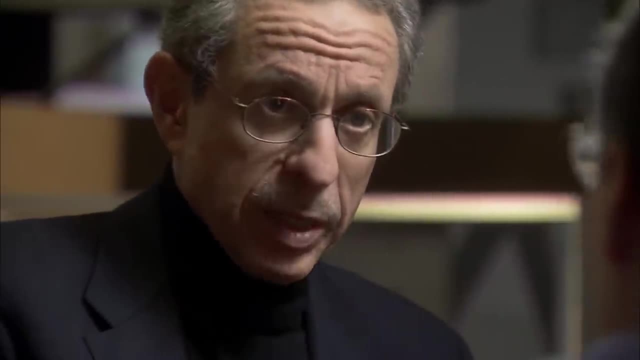 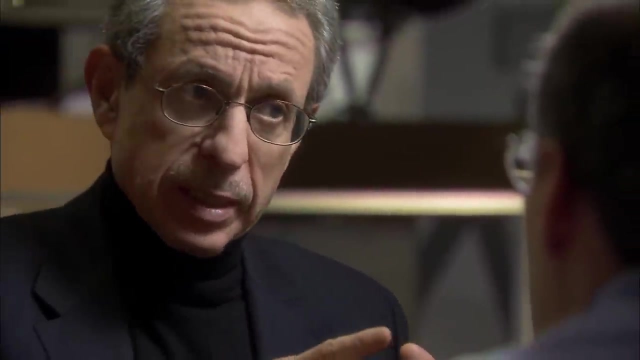 at the very beginning, after the cosmic microwave background picture had very little impact because it was much smaller, but over time it's growing in its impact. so it didn't affect very much the early structure Precisely And in fact, if dark energy had been, 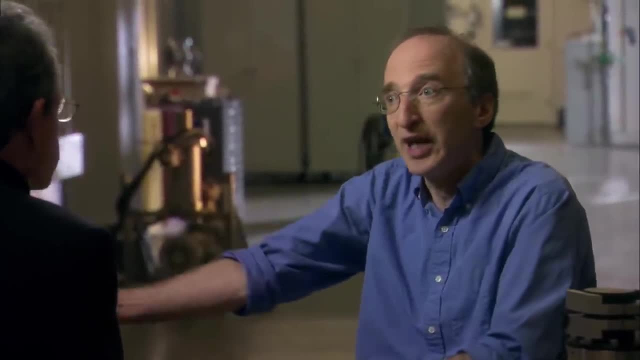 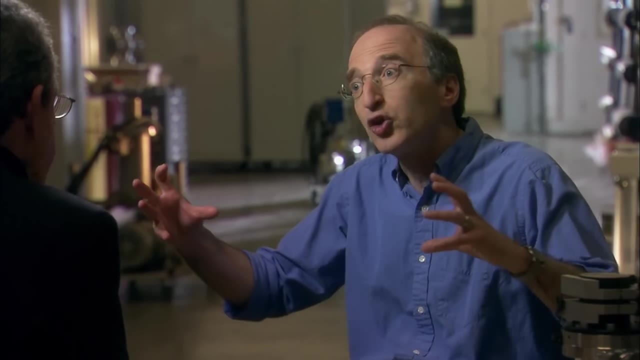 a much more important part of the universe. in the early days you would have ended up, you know, in a very different world than we see around us. It would have expanded things so much that nothing could have clustered and we would not have the galaxies. 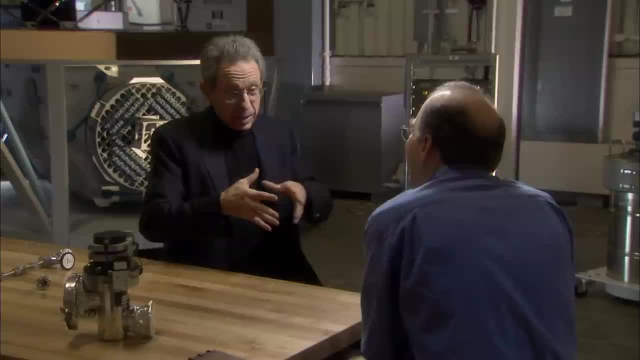 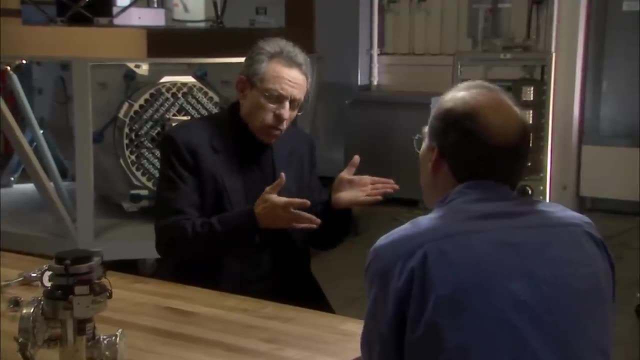 and clusters of galaxies and us that we see today. Yeah, so we like the dark energy in a sense to make things the way they are today, but if it started too soon or too strong, it would have Precisely. 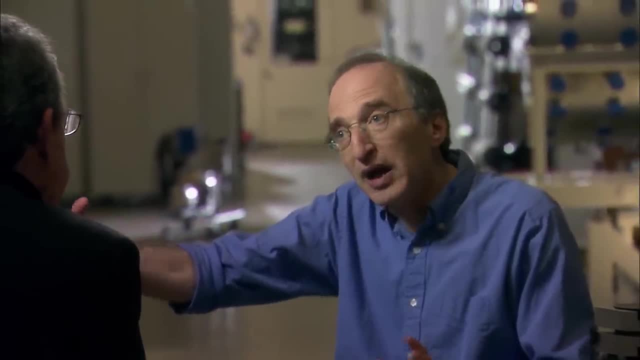 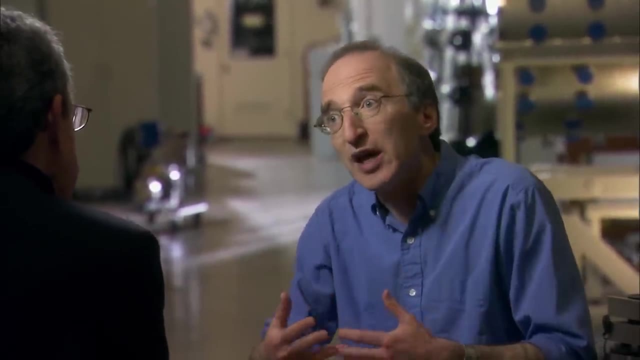 There'd be nothing here. What is the time frame? Typically, in the current picture, it's half of the universe: the first you know, 7 billion years approximately, and the most recent 7 billion years. it became so dilute that the dark energy took over. 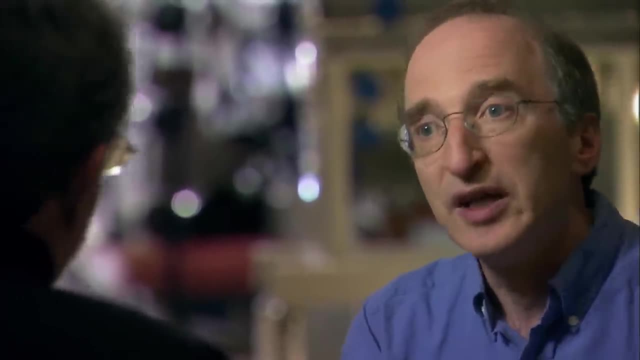 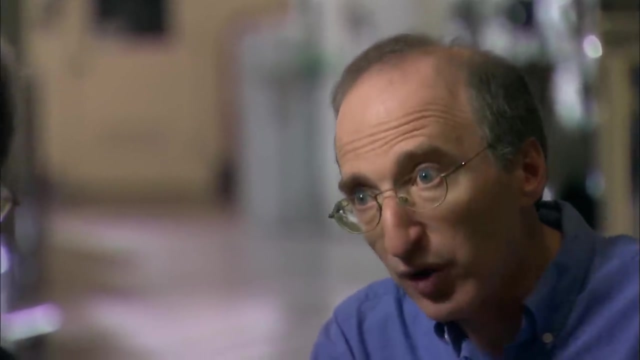 and started to accelerate the expansion. So it's real. its strong effect is after it starts to kick in and then it stops. it slows the clustering down, but during that same time period, while our sun and earth and solar system were forming, 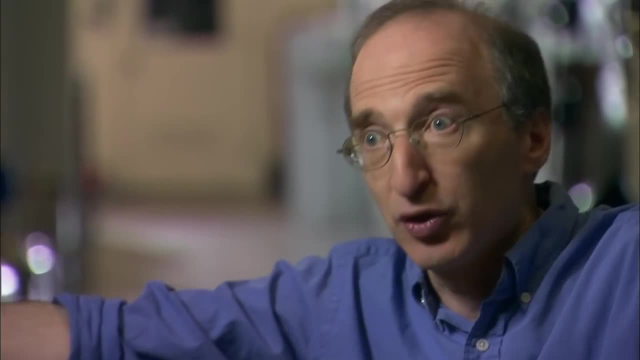 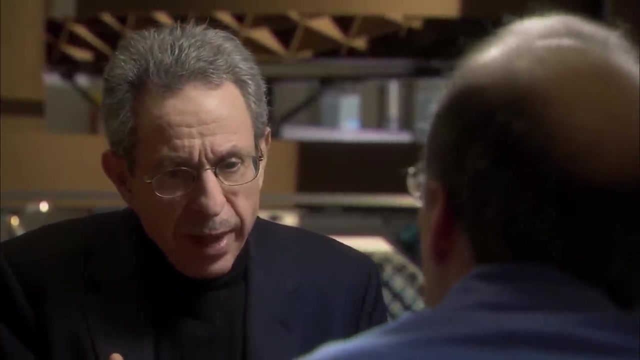 it was having an effect on how clustering was happening of large-scale things in the universe, like clusters of galaxies. So it's underneath what this dark energy may be, and so, as our theories develop, is it possible that whatever is causing that might be more complex than we realize? 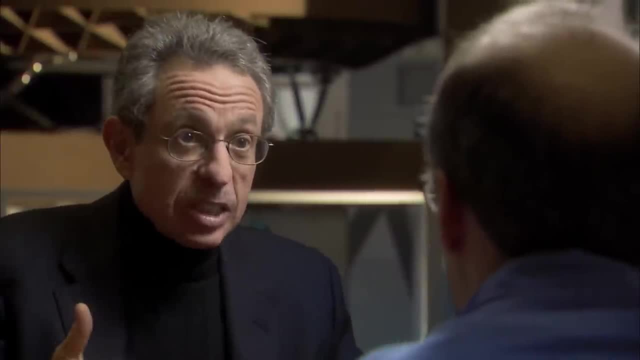 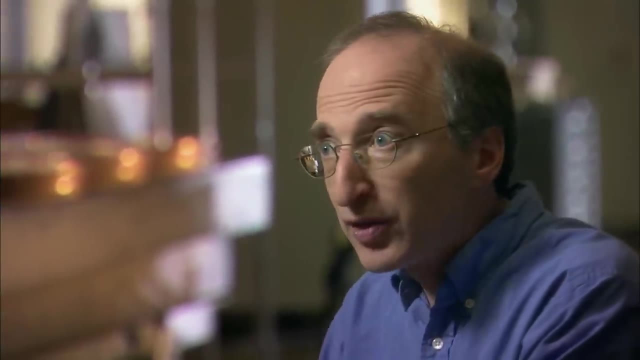 and as we tease apart the elements, it could lead to an even greater understanding of how the large-scale structure developed. Oh, I mean absolutely, And I should mention that when we say dark energy, that's sort of almost loading the question. 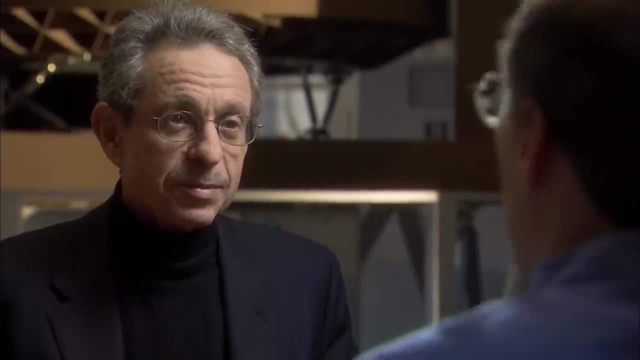 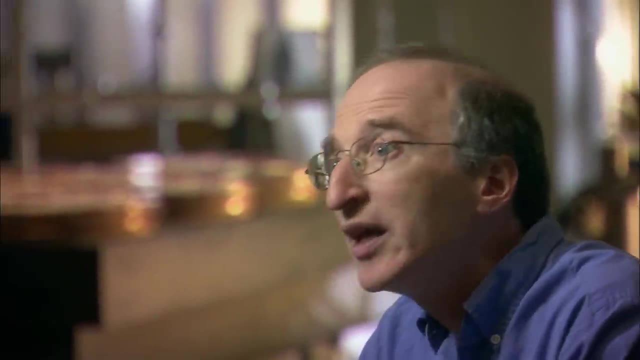 It almost makes it sound as if we know that the answer to what's causing the acceleration is an energy pervading all of space. It's perfectly possible that what we'll find is that we just don't have a quite sophisticated enough equation or theory of gravity. 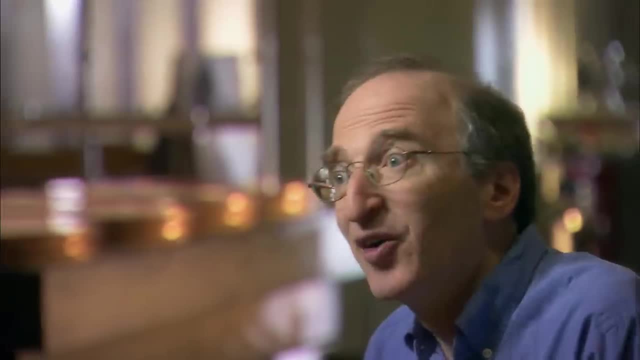 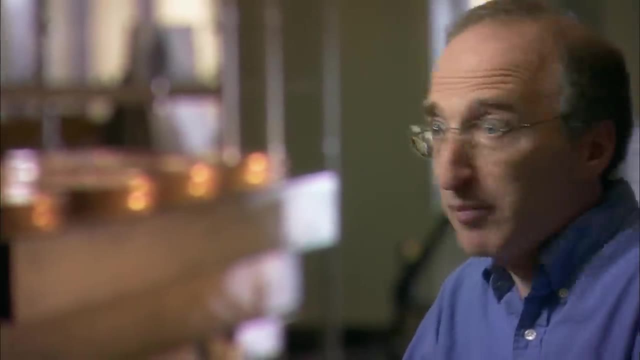 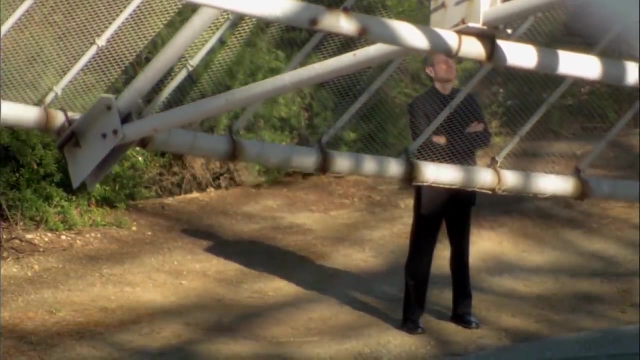 and that would be a huge discovery if it turns out that if we can slightly modify Einstein's theory of general relativity and explain this acceleration, it may allow us to explain many other things that we otherwise will never get to. Throughout history, humans have pondered cosmology. 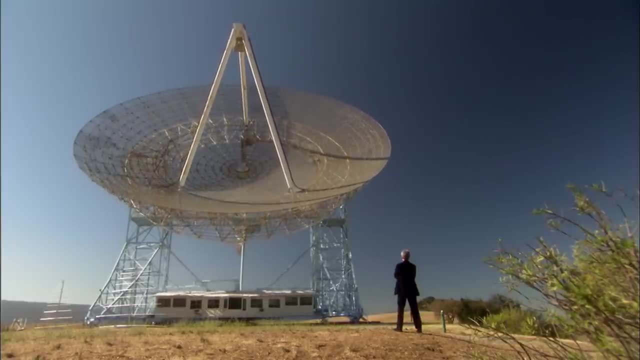 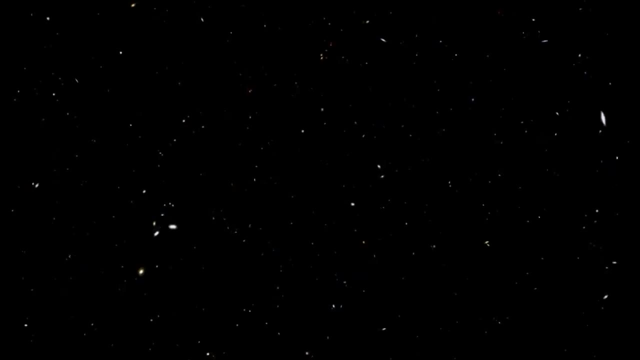 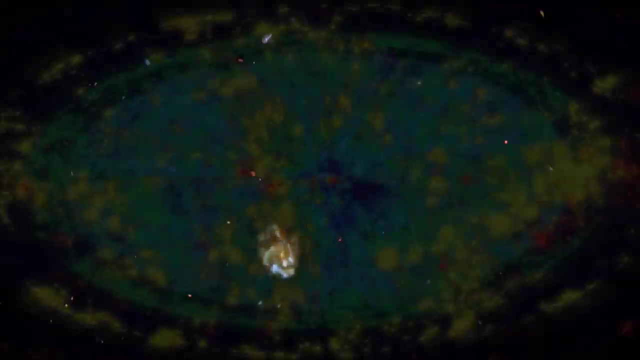 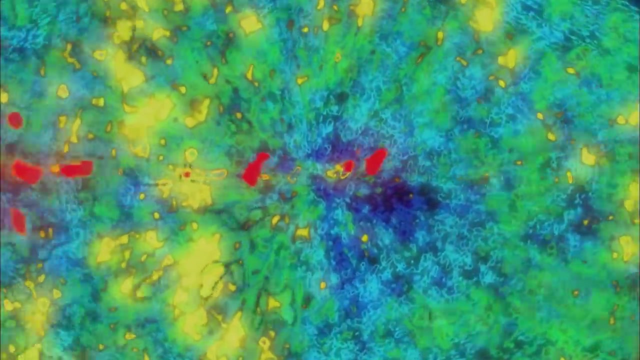 the origins and ends of the universe, Immense questions traditionally commandeered by religion and philosophy. One of the magnificent achievements of science is the transformation of cosmology into a precision science. The discoveries are astounding: The cosmic microwave background radiation providing a baby. 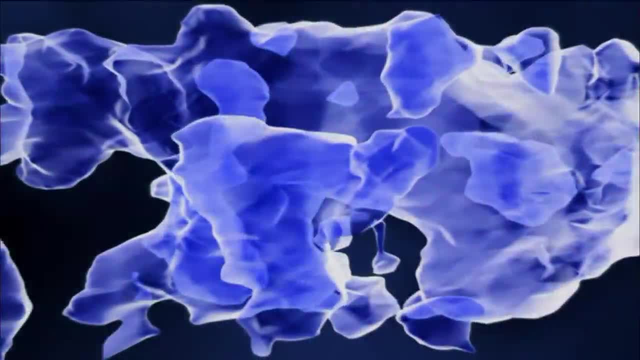 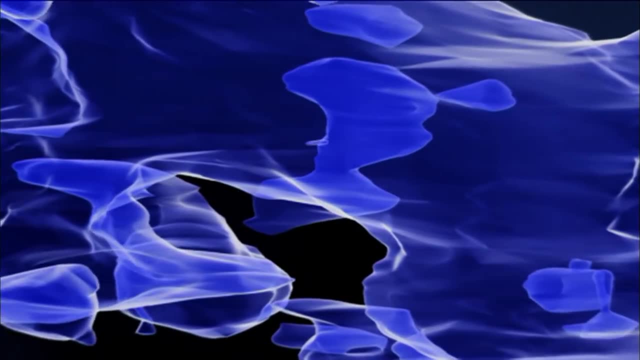 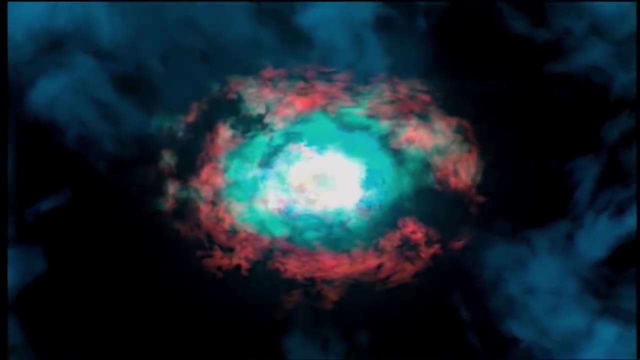 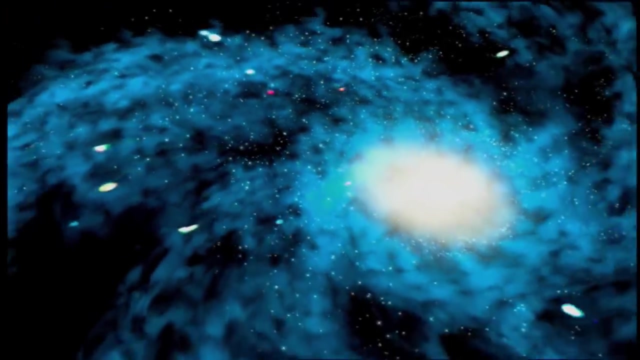 picture of the early universe. Dark energy, its increasingly strong repulsive force expanding the universe and determining its fate. Quantum fluctuations buried deep within the universe's first micro, micro, micro, micro, microsecond, providing all the seeds for all the billions of galaxies. 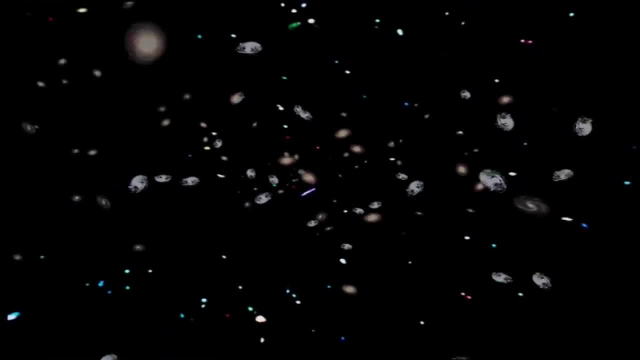 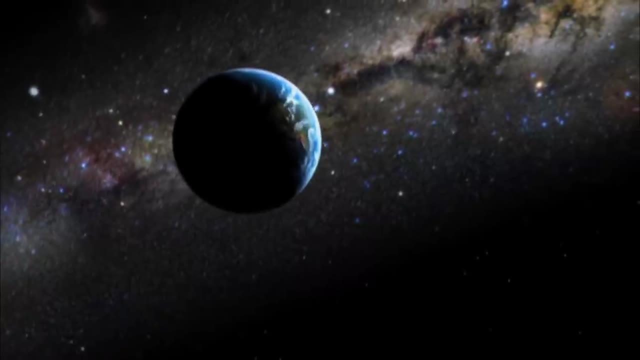 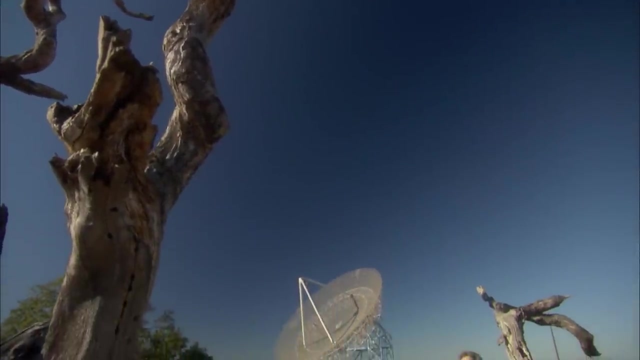 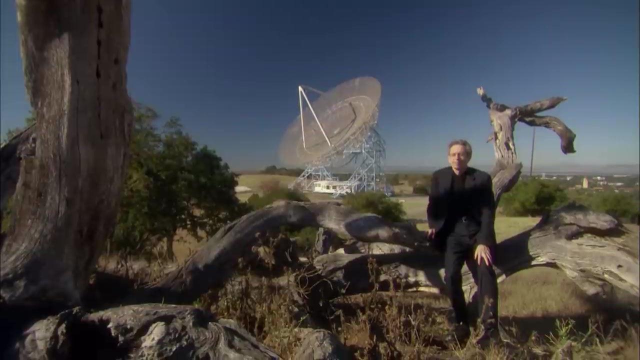 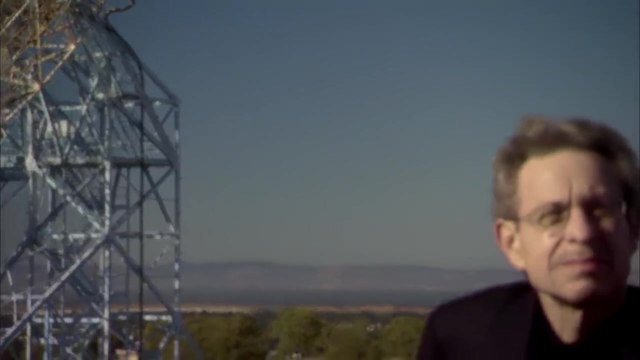 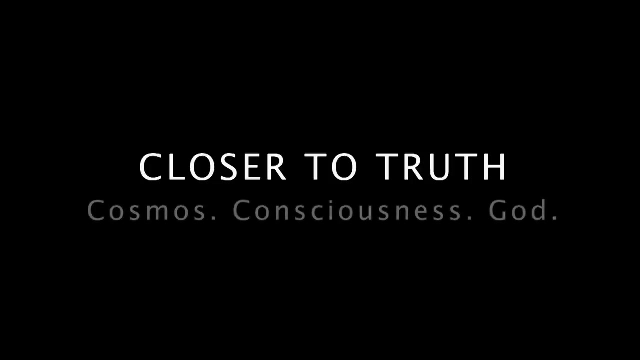 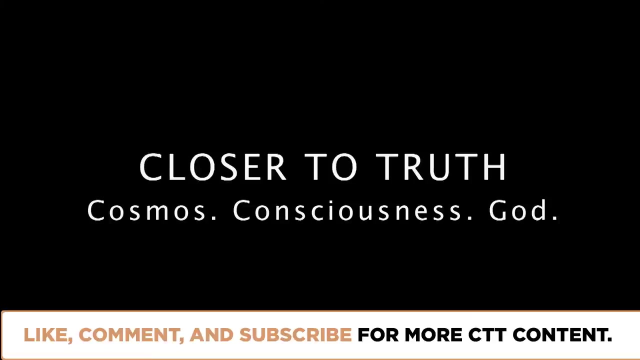 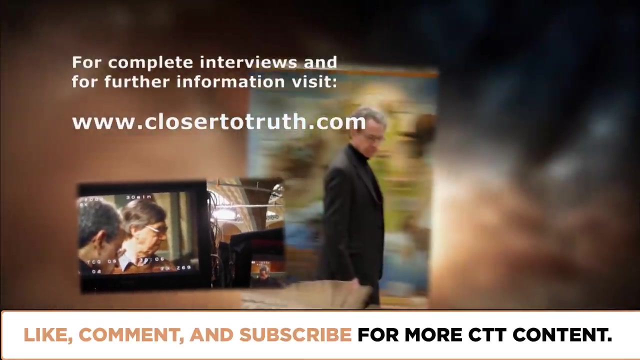 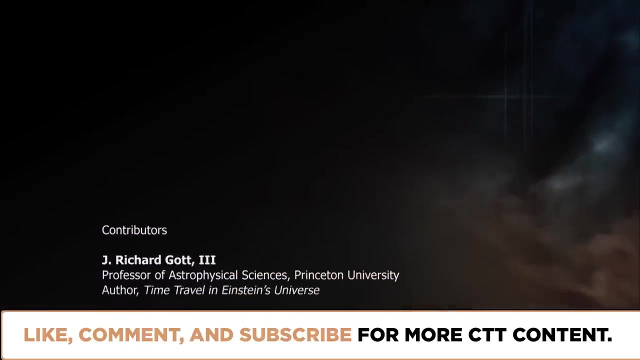